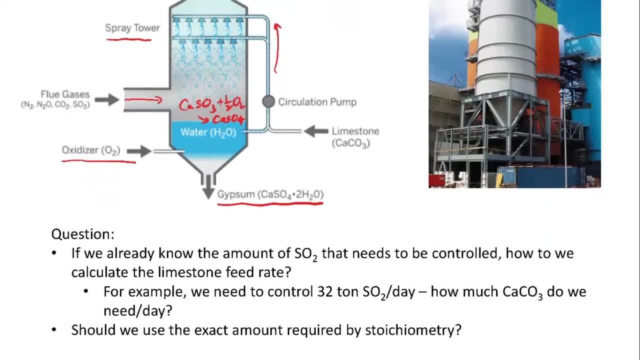 So we also mentioned a few questions, right? So if we already know the amount of sulfur dioxide that needs to be controlled- similar to the problem or the team project you're working on right now- So, based on the co-composition, you can calculate how much sulfur dioxide you can generate from this combustion process? 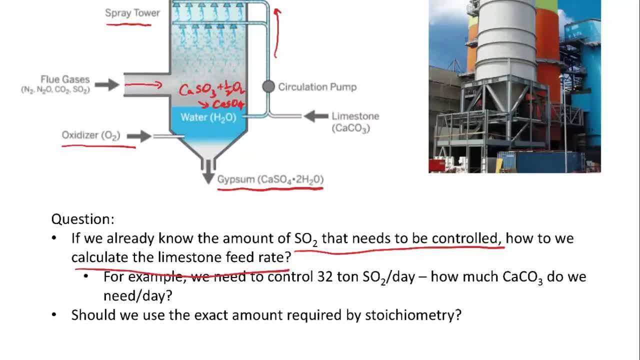 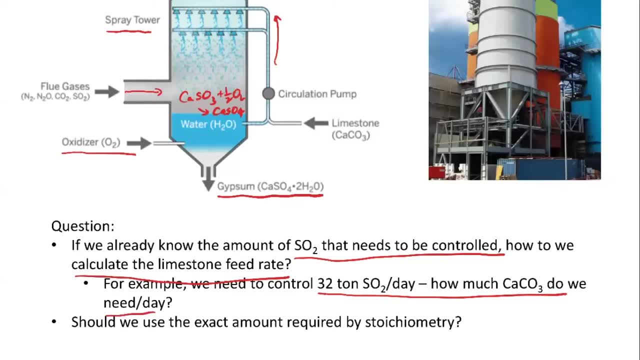 Then how do we calculate? How do we calculate the limestone feed rate? Okay, so here I'm listing this question again, So we briefly introduced that in our last class. but let's here do a quick calculation. Launch of quiz. So if we know that we need to control 32 tenths of sulfur dioxide per day, 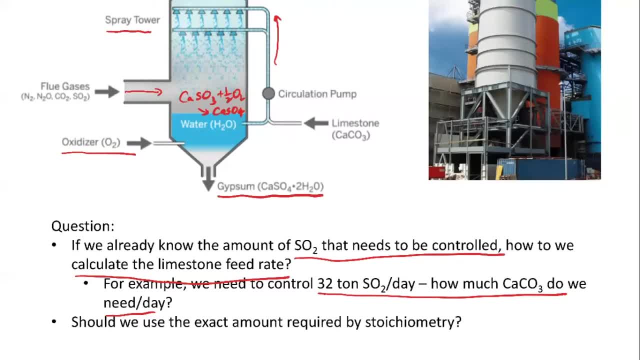 then how much calcium carbonate do we need to feed? So that's what we interested in, is the question here. So how many different types of carbonate do we need to feed? So we are using one carbonate per day per year, and the other carbonate we need to feed is one carbonate per year. 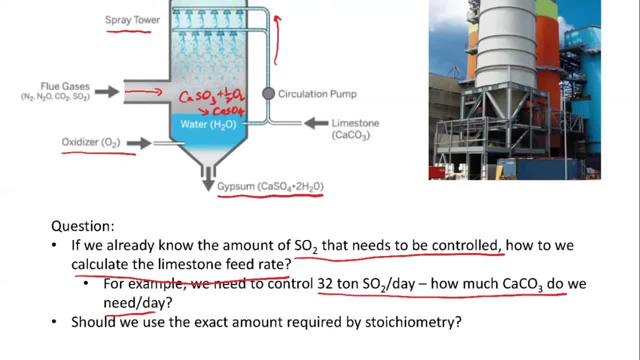 And then we will use another carbonate per year. So this is what we call a carbonate per year. Let's see? Okay, 10 more seconds. Okay, we'll stop here. So the correct answer is 50 tons per day. So we give a very simple solution to this question. 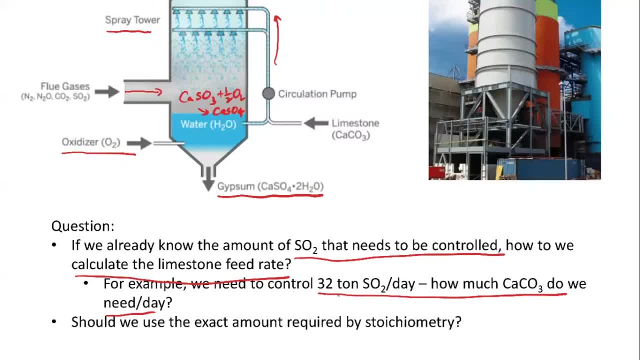 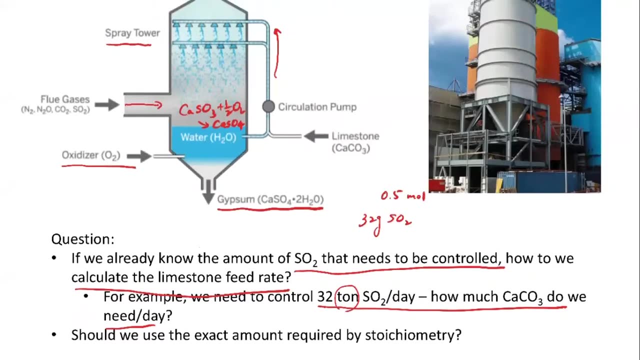 So we're assuming that first. let's not look at the tens here. Let's assume that there are 32 grams of sulfur dioxide. So 32 grams of sulfur dioxide means it's point five moles of sulfur dioxide, right? And we know that sulfur dioxide react with calcium carbonate. 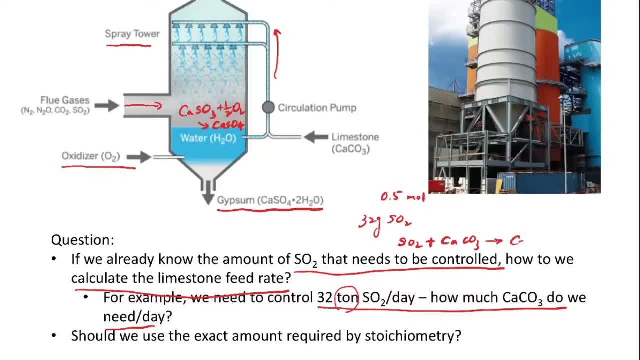 At a one to one ratio. So we form calcium sulfate and sulfite and carbon dioxide, right? So they're at a stoichiometric ratio of one to one. So what that means is, if we want to neutralize point five moles of sulfur dioxide, then we 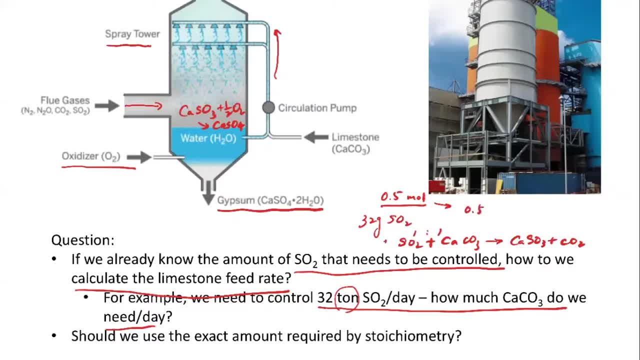 need point five moles of calcium carbonate. okay, So the molecular weight of calcium carbonate is 100, 100 gram per mole, right? So what that means is we need 50 grams. So 32 grams of sulfur dioxide needs 50 grams of calcium carbonate, right? 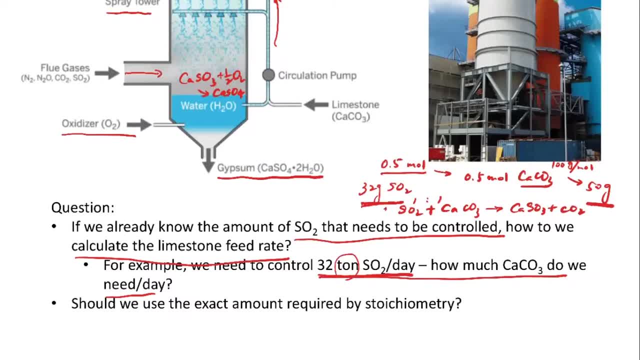 So that's why 32 tens of sulfur dioxide needs 50 tens. okay, So this is a very simple solution, Okay, Okay, So this is the stoichiometric ratio question. So if we know which molecular ratio they're reacting, then we can calculate. we should. 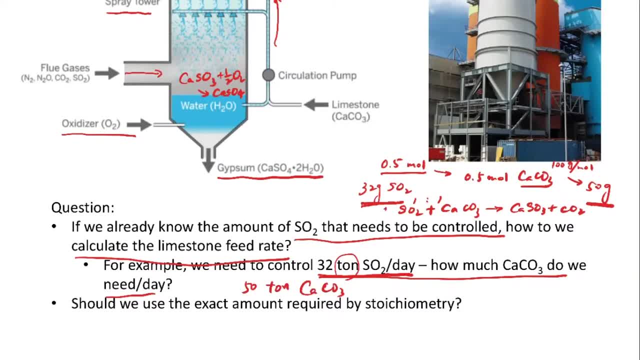 be able to calculate how much of the calcium carbonate we need- And this is the general question we're going to face- for the sulfur dioxide control or the either the wet scrubbing or the dry scrubbing process. So we're interested in two questions. 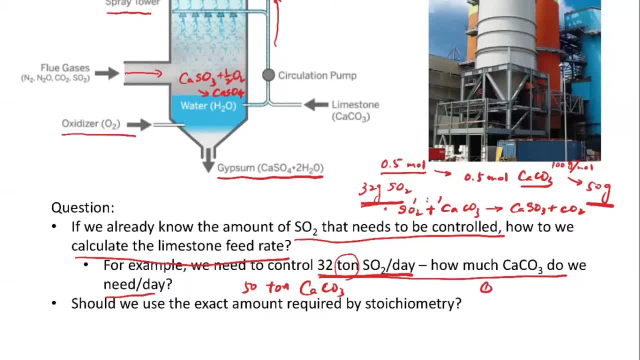 So the first question is: how much, How much raw material you need to feed Right, For example, how much limestone we need. And the second question is: how much slurry will afford? well, will form, how much sludge right? 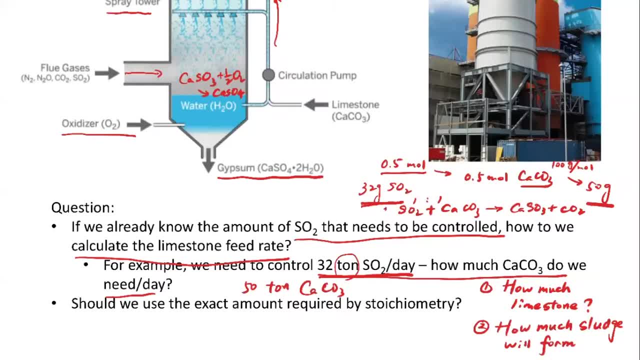 For the sulfur dioxide design. Right, Yeah, Okay, sulfur dioxide control design. we're mainly interested in two questions. One is: how much limestone should we feed into the system? Either limestone, lime or trona, all the raw material that can neutralize. 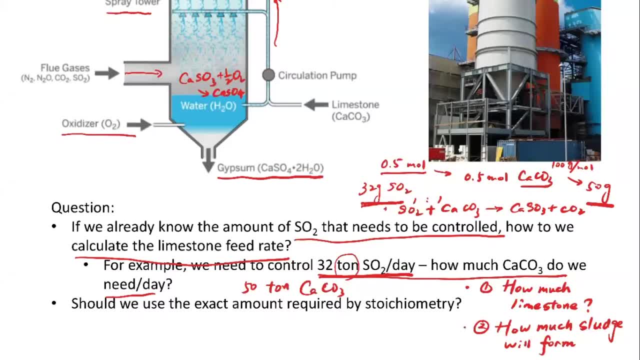 these acidic gases right? And the second question is how much product we're forming, because finally we need to transfer this product to somewhere else. If we don't know the quantity or production rate of this product, then we cannot design the system right. 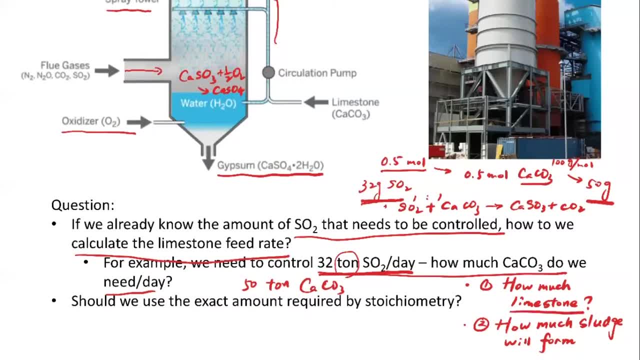 So here the limestone is a raw material or the reactant. The sludge is basically what forms at the bottom of this reactor, right? So it's going to be composed of water, going to be composed of calcium sulfate, right? And then, of course, the reaction is not complete generally. 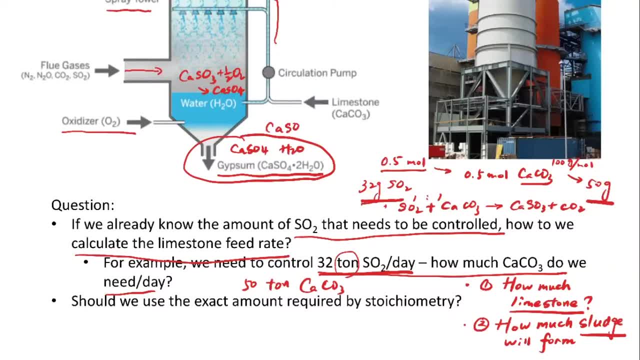 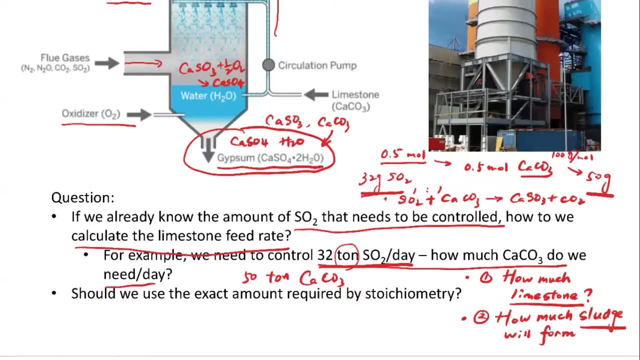 So there are still going to be some calcium sulfate that's being remained, or the calcium carbonate, right? So the sludge is going to be a mixture of all of these chemicals. okay, So these are the two general questions and we can use the similar idea. 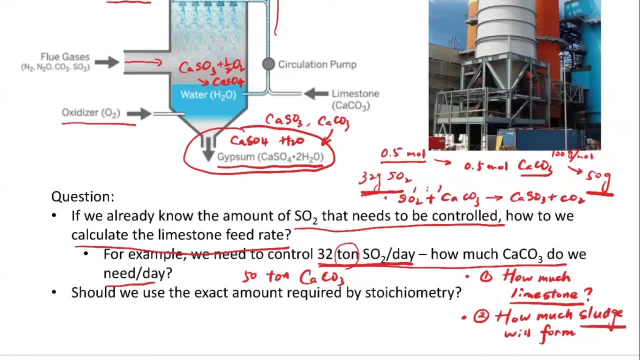 to understand what is happening here. So let's say, right now, we assume that 32 tenths of the sulfur dioxide is being neutralized. What that means is that we need to provide 50 tenths of the calcium carbonate. right, So we're going to put 50 tenths of the calcium carbonate. 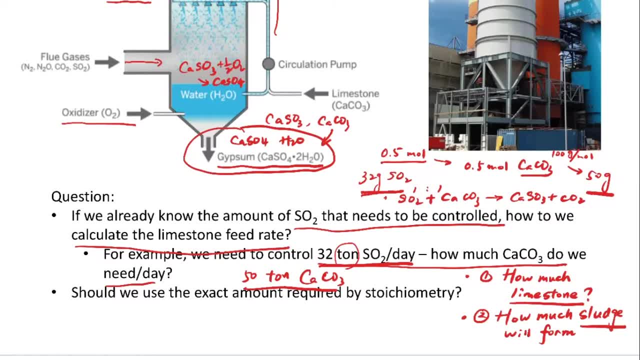 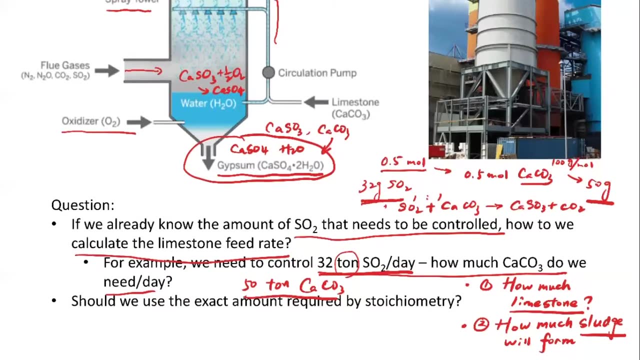 into the system. But unluckily the limestone is not purely composed of calcium carbonate, So there is always some impurities in the limestone there. So there are going to be a little bit more complexity. And let's for now, if we assume that the limestone 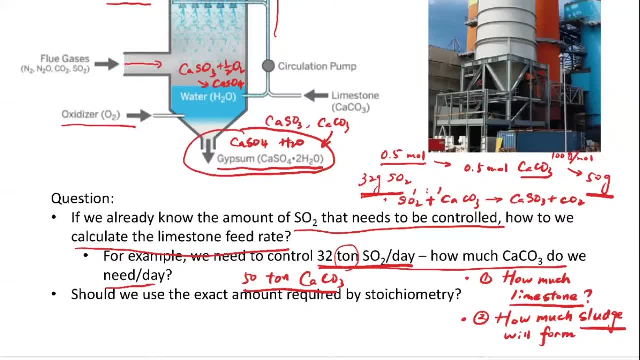 is purely composed of calcium carbonate, then based on this relationship, then we can calculate how much of the calcium sulfate we're going to form from this process. right, We know that everything is reacting at a stoichiometric ratio of one to one. 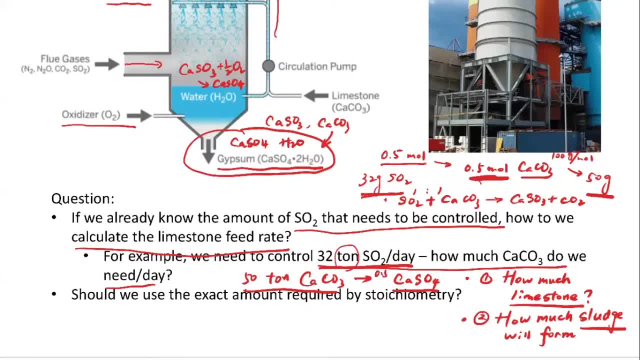 So what that means is we're going to form 0.5 moles of the calcium sulfate, right, And then, if we know the calcium sulfate mass, then we can calculate how much of the sludge we're going to need. okay, 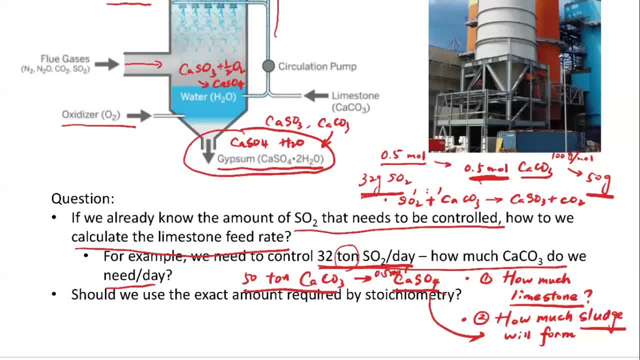 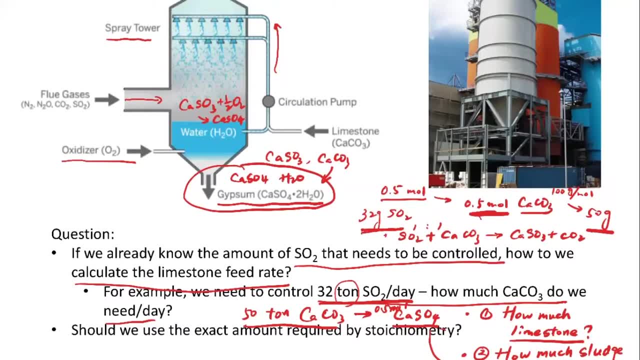 So everything is still based on the stoichiometry, but due to the impurities, the impurity of the limestone, and also when you always need to provide, basically provide more limestone into the system to completely neutralize these acidic gases. So the situation will get a little bit complex. 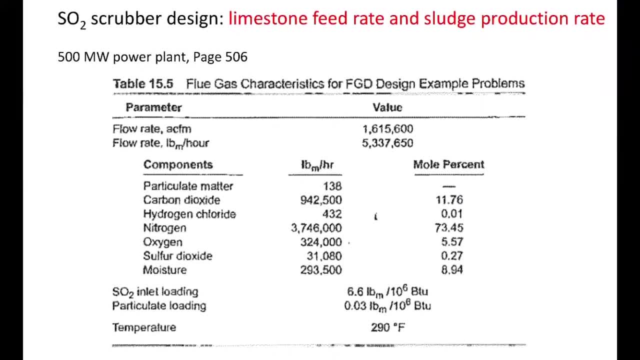 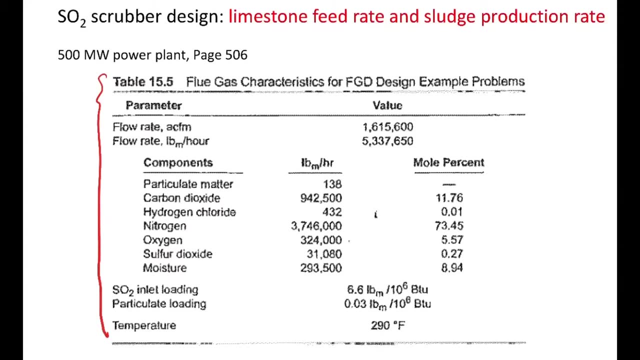 So here, what I'm showing is an actual design system. So I mentioned in our last class that in your design problem or team project, you also need to come up with this table here, right, That will basically give an overview of what is the composition of the flue gas. 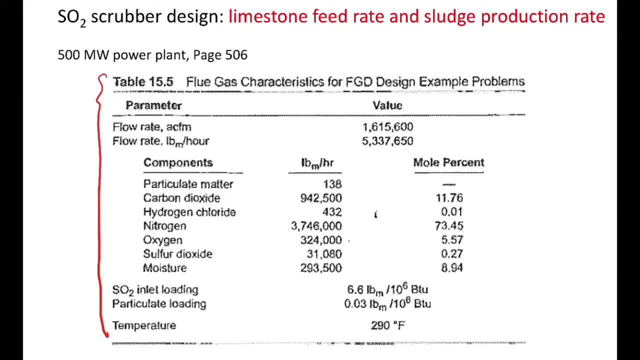 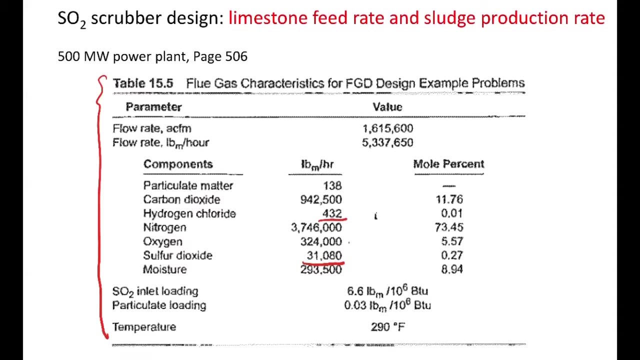 from this co-combustion process right, And then further, based on the composition of the sulfur dioxide and hydrogen chloride, we should be able to calculate what is the limestone we need in the entire system. okay, So again I'm listing the two questions. 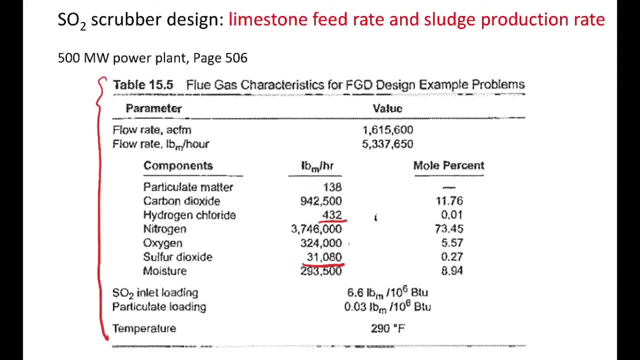 or the two problems for this sulfur dioxide scrubber design problem. So the first is the limestone feed rate and the second is the sludge production rate. okay, So these are the two questions that we have to deal with. So, under actual situation, 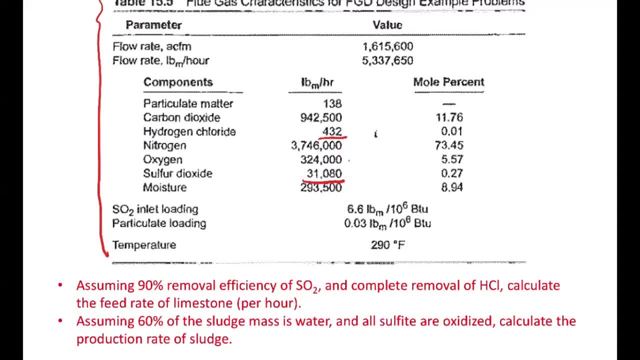 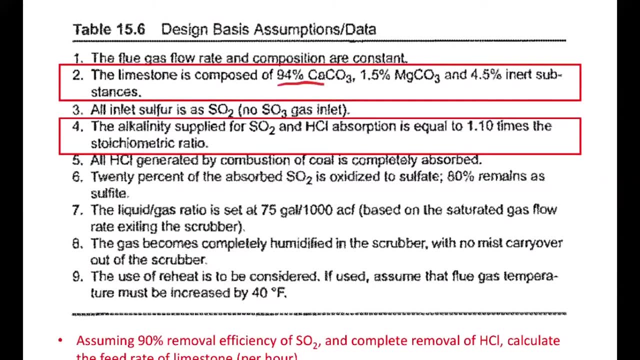 we cannot assume that the limestone is pure calcium carbonate anymore. okay, So if you look at the composition here, the limestone is generally composed of 94% of the calcium carbonate, 1.5% of the magnesium carbonate and there are some inert materials. okay, 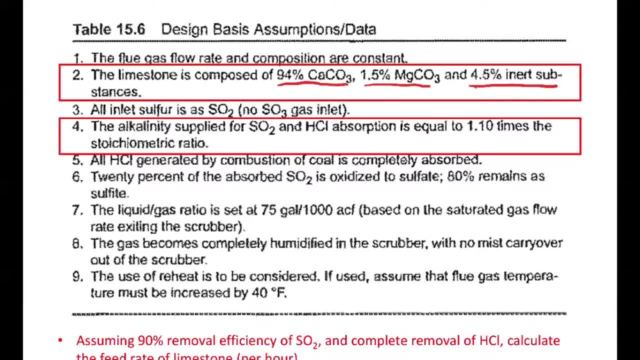 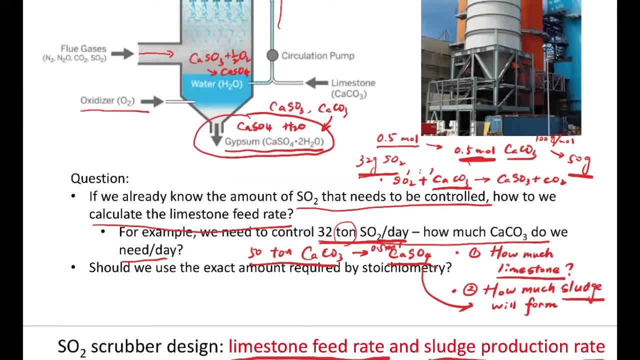 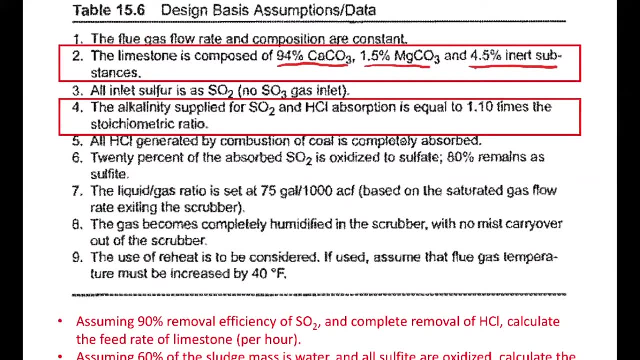 But this shouldn't affect the solution a lot, because we're not letting these acidic gas to react with calcium carbonate. We're actually letting them to react with the carbonate ions, right? So it doesn't matter whether it's calcium carbonate or whether it's magnesium carbonate. 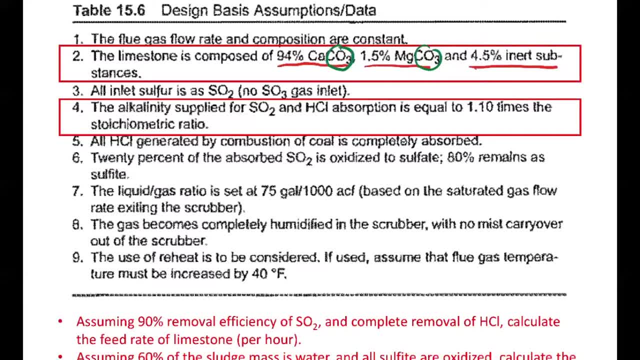 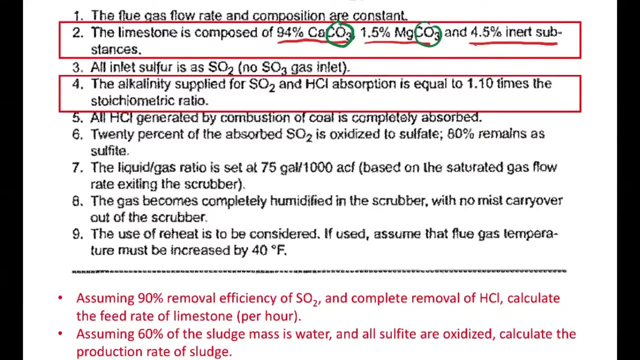 So as long as we know what is the carbonate it needs for this neutralization process or neutralization reaction, then we should be able to relate that to the limestone. okay, You see? the second point is that generally, we'll provide more limestone into the system. 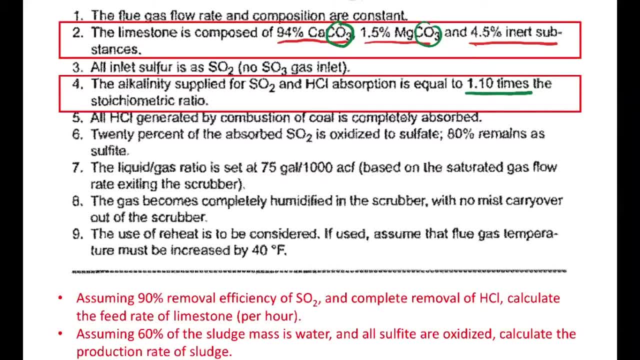 which is 1.1 times of the stoichiometric ratio. right, Basically, we'll provide 10% more of the limestone into this scrubber so that it can more completely react with acidic gases, right? So let's say that we further assume. 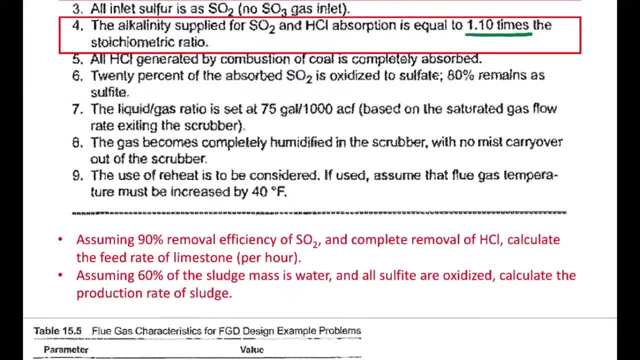 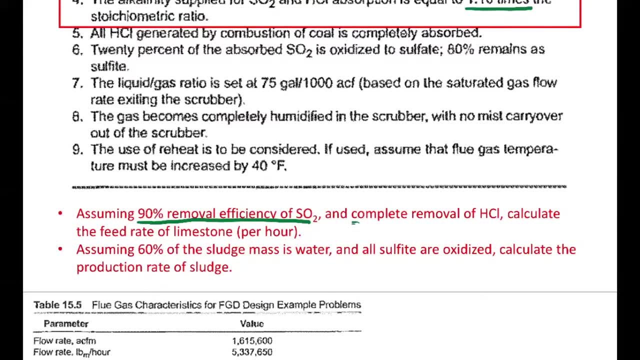 that the removal efficiency of the sulfur dioxide is 90% And for the hydrogen chloride there is a complete removal. Okay, so these are the assumptions that were made onto this reaction here. Then let's say: how do we calculate the feed rate of the limestone? okay, 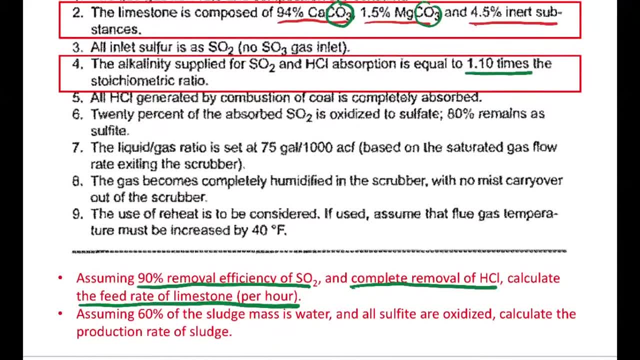 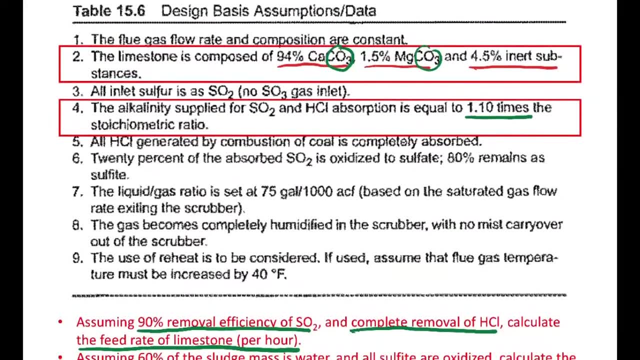 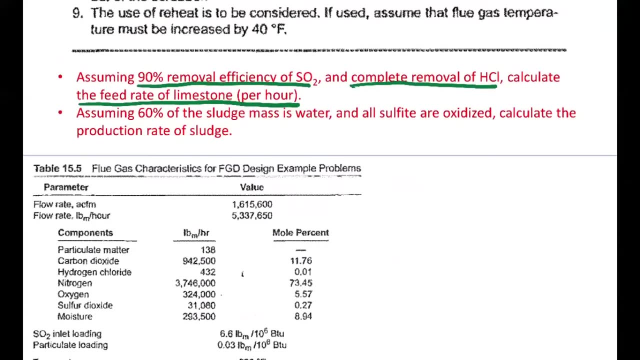 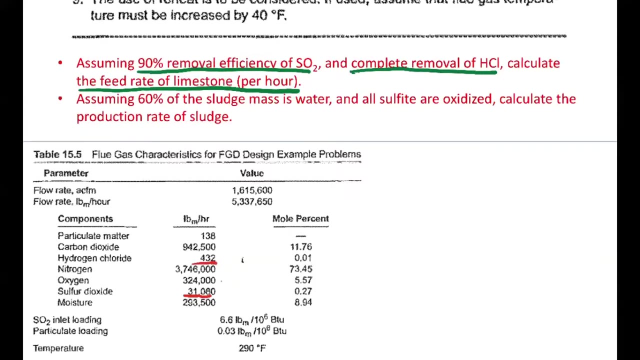 The foot rate would be 90%. The solution would be 90xos. Let's say that we can。 That rise will be 2.6.. That fall will be 2.4.. The soil would be as simple as 10 when we measure the放 Бог. 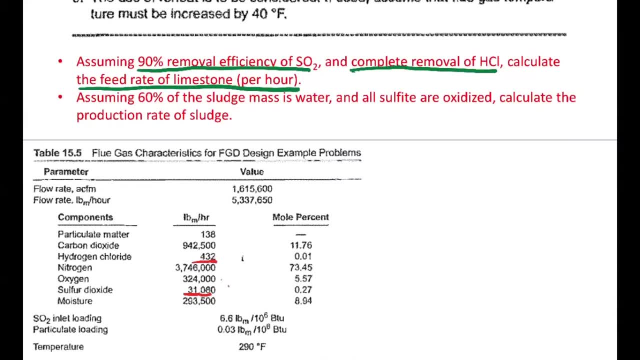 And for this Kirchhoff's we get a constant elevation right. Correct, assume that we just removed 90% of the sulfur dioxide here, But here for the hydrogen chloride we remove 100% of them And then basically these acidic gas. 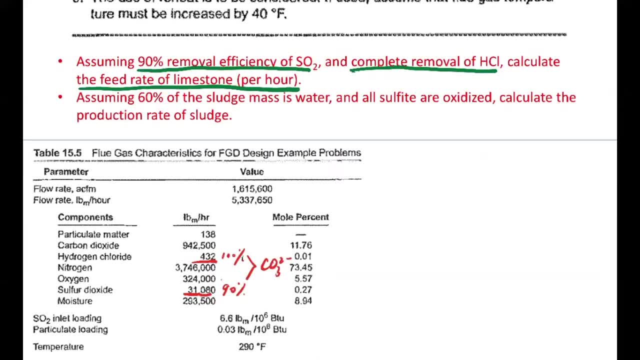 will react with the carbonate ions and basically get neutralized, And these carbonate ions are being provided by the limestone, And we know that the limestone is further composed of calcium carbonate, magnesium carbonate and inert. So the question is asking us what is? 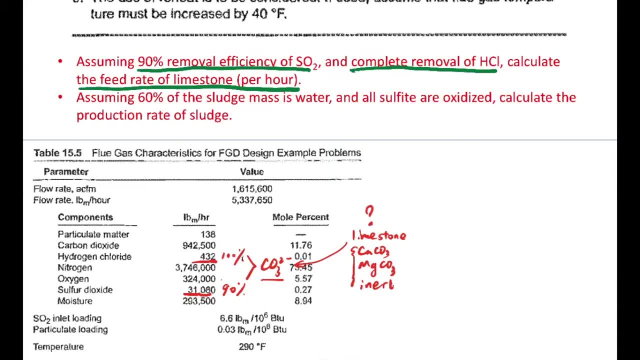 the feed rate of the limestone. So maybe we can put some thoughts on this and look at this problem for maybe one minute or two minutes, and then we can start to discuss this. All right, Thank you. OK, I think we can. 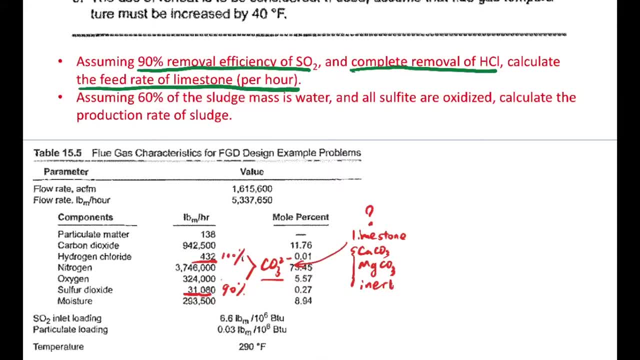 We can start to analyze this problem, All right. So for these sulfur dioxide control design problems, we need to understand what is our target and what is the reality. So, basically, the target is to neutralize these acidic gases. All right, And we know that. for these sulfur dioxide control design, 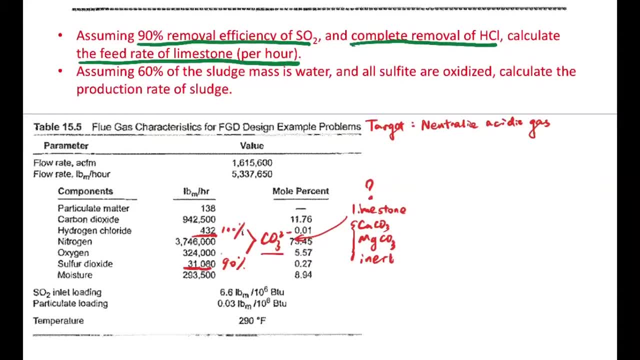 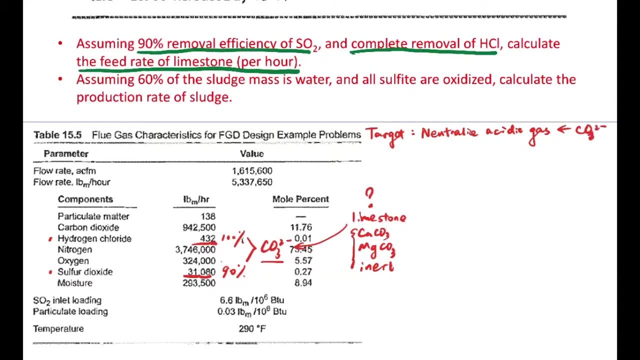 problems. for this problem, we need to neutralize hydrogen chloride and sulfur dioxide, OK, And we're trying to use carbonate ions to neutralize these species, OK. So that's why, in order to calculate the limestone feed rate, or the amount of limestone we need, 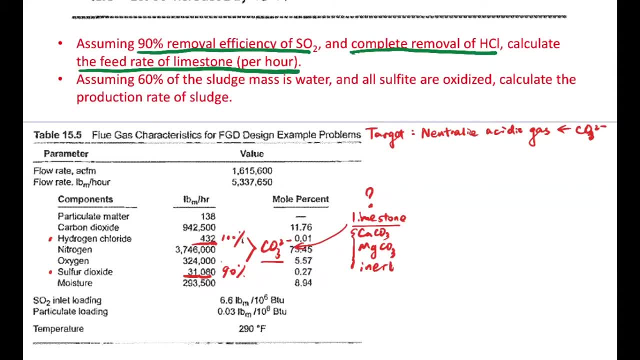 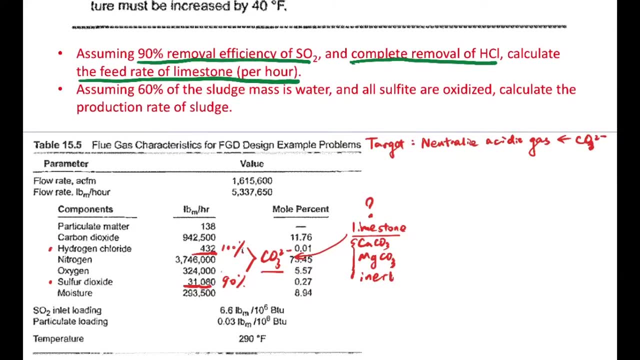 we need to first know what is the amount of the acidic gas. OK, So for this problem there are already a lot of things We can already provide you. what is basically? what is the flow rate or the rate of generation for these acidic gases? 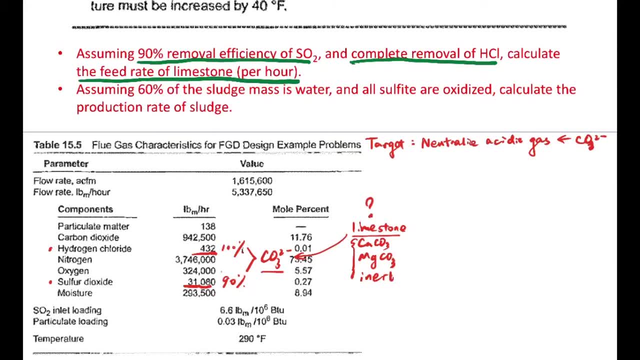 We can quite easily calculate that, And you notice that here the units are in the US units or the British units, Right? So for simplicity, let's convert it to the standard units first. OK, So basically we can calculate what is the flow rate of the sulfur dioxide. 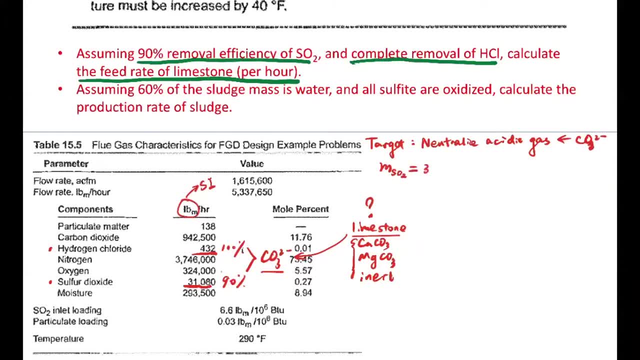 OK, So that's 31.080.. And then our goal is: we want to neutralize 90% of them, right? And we'll convert this into kilograms, which is 0.45.. So it's kilogram per pound. 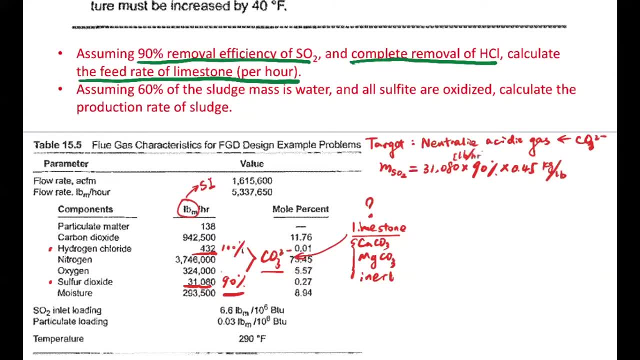 And then here the unit is pound per hour. OK, So that's 1,, 2,, 5,, 8,, 7.4 kilogram per hour. OK, So if you have a calculator, I think now is also. 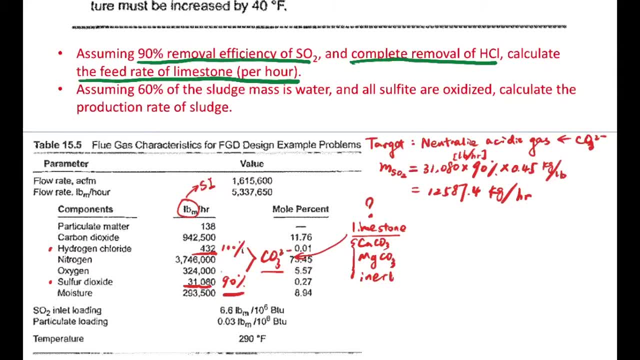 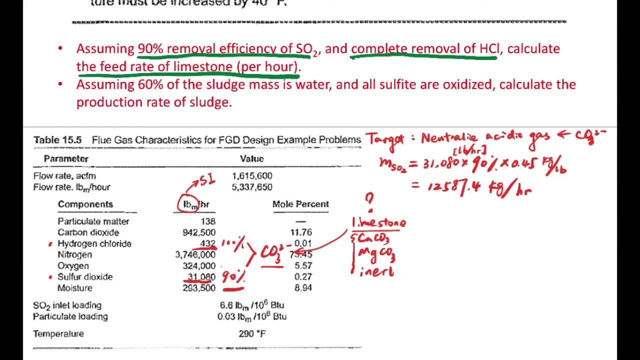 a good time to check whether these answers are correct. Right, So this is the amount of the sulfur dioxide we need to control. I mentioned that it's being reacted at a rate of efficiency of 90%, Right, OK, Right, And then we also need to control the hydrogen chloride, which 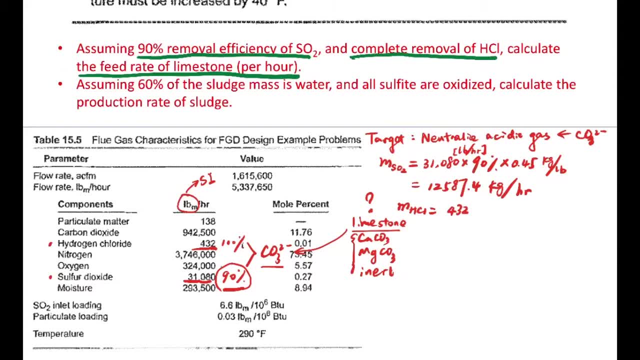 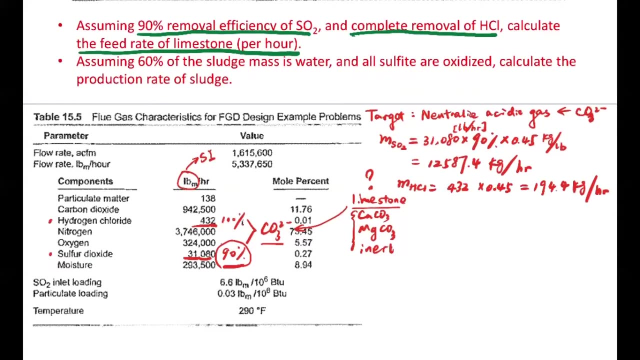 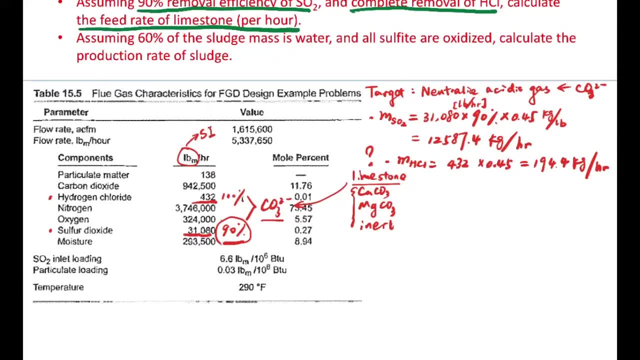 Right. And then we mentioned that to neutralize these acidic gases we're using carbonate ions, Right? So, based on their mass flow rate, we should be able to calculate what is the molar flow rate of the carbonate ions it needs for the reaction. 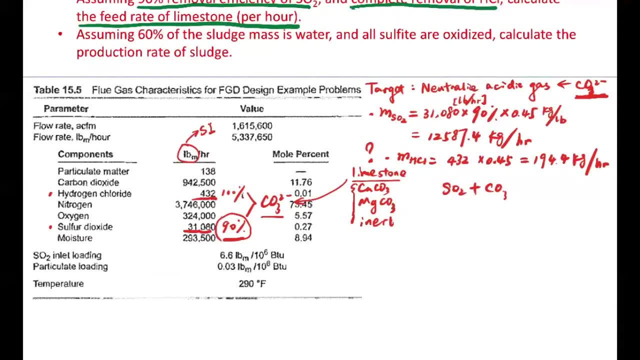 Right. So we know that the sulfur dioxide reacts with the carbonate ions at a stoichiometric ratio of one to one, because we're forming sulfide ions- carbon dioxide right- And then two numbers of hydrogen chloride will react, one number of the carbonate ions. 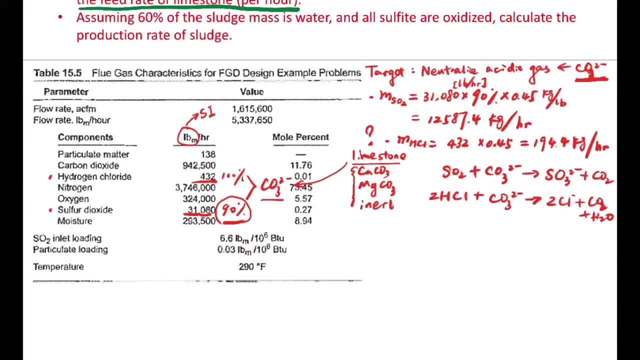 Okay, so this is a reaction for the hydrogen chloride and the carbonate ions, So we have these two reactions. So what this means is that, in order to neutralize one mole of the sulfur dioxide, we need one mole of the carbonate ions. 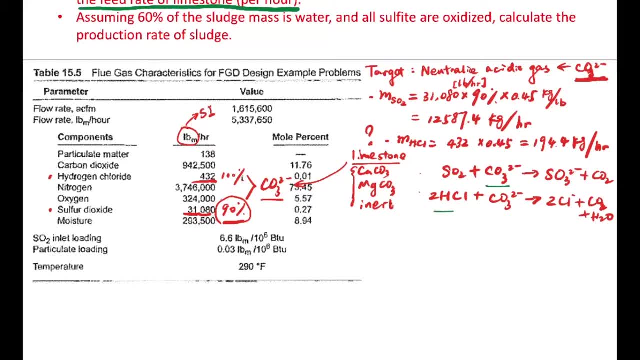 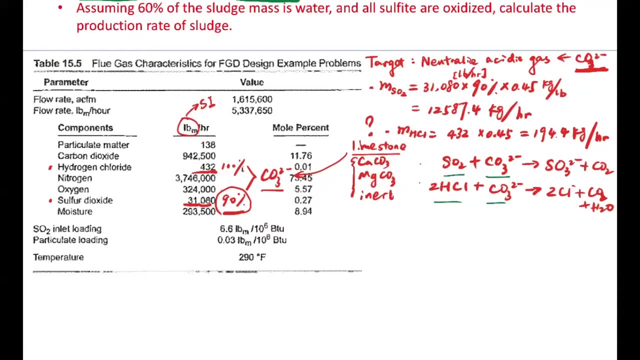 And in order to remove one mole of the hydrogen chloride, we just need 0.5 mole of the carbonate ions. right, And since we already know the mass, we can calculate what is the carbonate ions it needs to remove these acidic gases. okay, 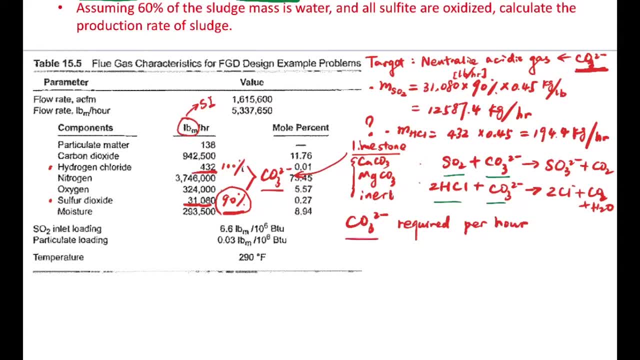 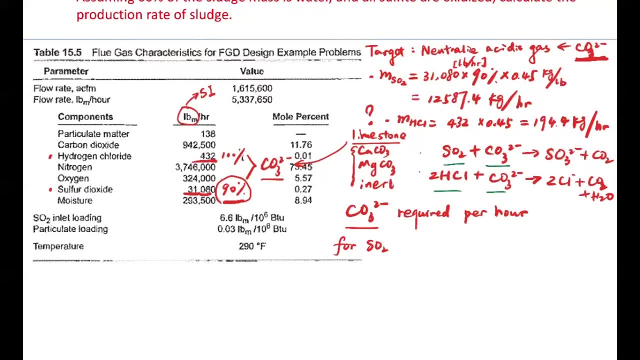 So we can calculate what is the carbonate ions that it requires for each hour. So for the sulfur dioxide, and because of this reaction here, we know that it's going to be one to five. Let me list all the equation here, Right? 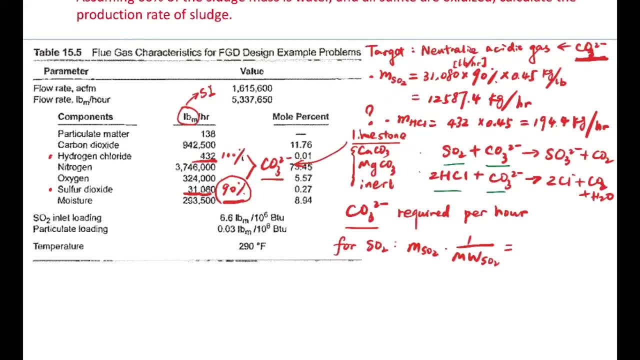 Simply because the sulfur dioxide reacts with the carbonate ions at a stoichiometric ratio of one to one. So the most that's required for the sulfur dioxide is just the mass flow rate divided by its molecular weight, right, So that's going to be one to five. 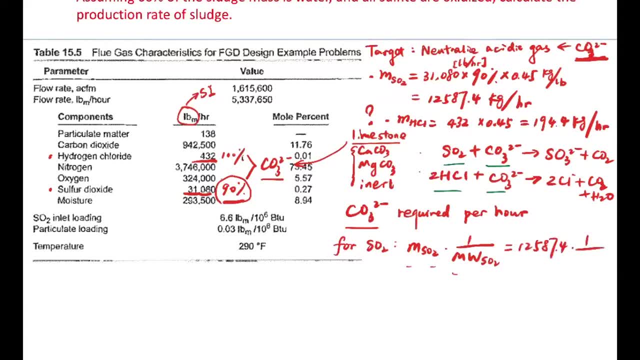 it's 7.4, divided by 64 grams per mole, So you can find out that this is 196, 671 mole per hour. So this is how many moles of the carbon ions we need to neutralize the sulfur dioxide. 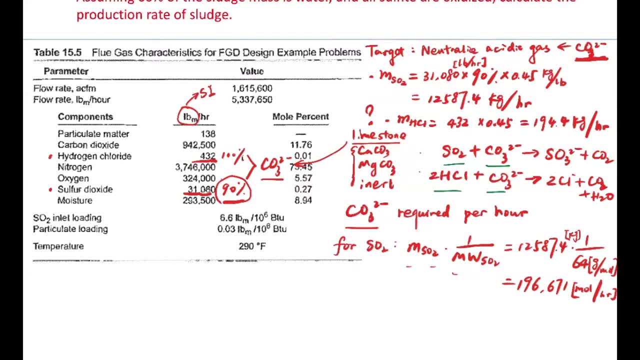 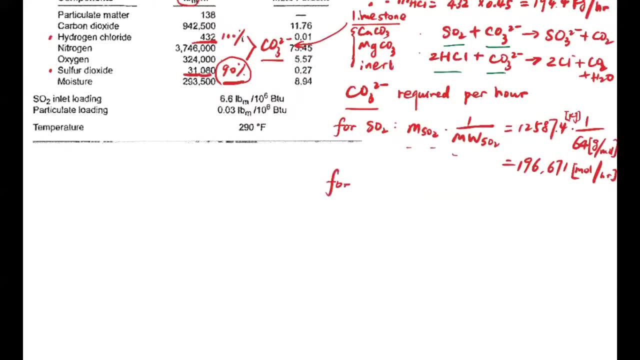 And this is what we get. So this is the amount of carbon dioxide that we need to neutralize the sulfur dioxide, Okay. And similarly, we can calculate this amount for the hydrogen chloride, which is MHCL, And then we'll divide this value by two. 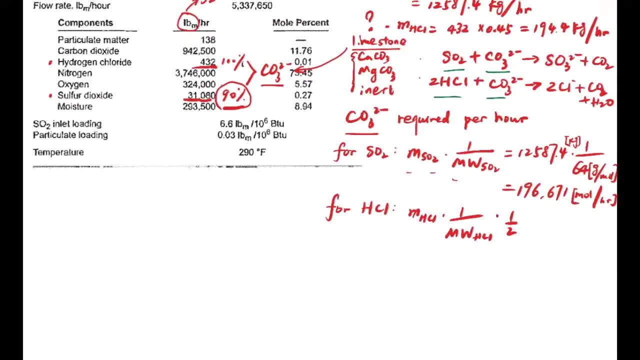 mainly because there's two moles of the hydrogen chloride will be able to remove, will be able to react with one mole of the carbonate ions. All right, so that's going to be 194 and four Okay. so basically based on the flow rate of the sulfur dioxide. 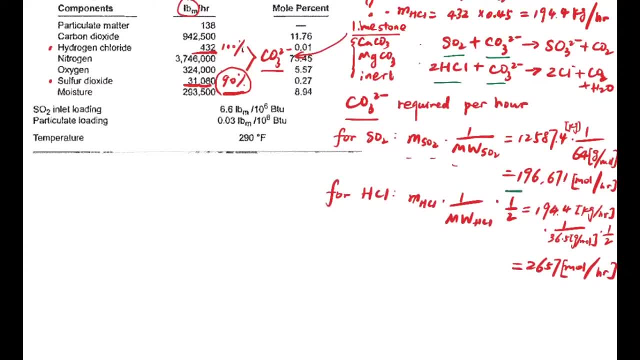 I'm going to be able to calculate the flow rate of the sulfur dioxide And hydrogen chloride. we can calculate what is the amount of the carbon and ions we need to neutralize these gas species. right, So the total required. let's say we'll move here. 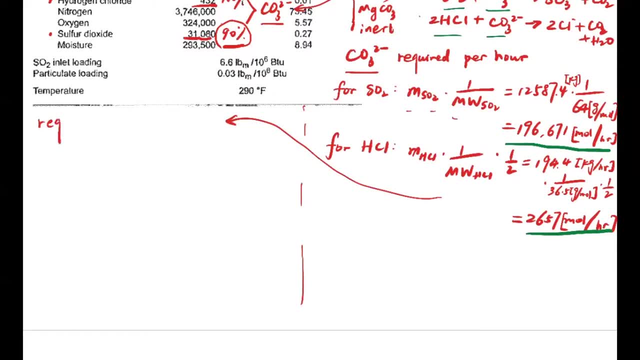 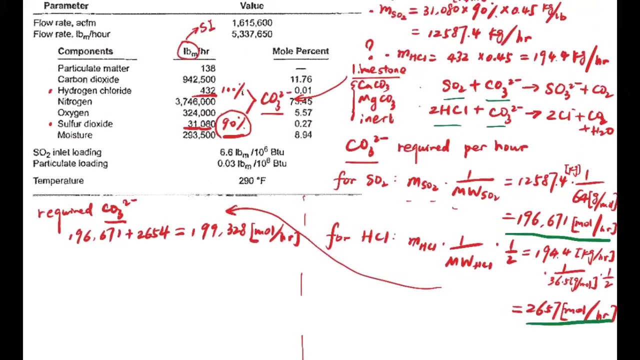 So the required carbon and ions is just going to be these two numbers added together. Okay, so this is the required carbon and ions. it needs to neutralize these gas acidity species And then, further in this problem, we assume that we will provide temperature. 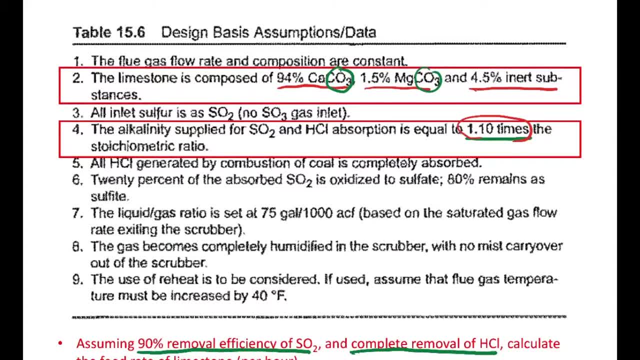 Okay, so this is the required carbon and ions. it needs to neutralize these gas acidity species. And then, further in this problem, we assume that we will provide temperature, So we need to provide 100% more of the limestone right. 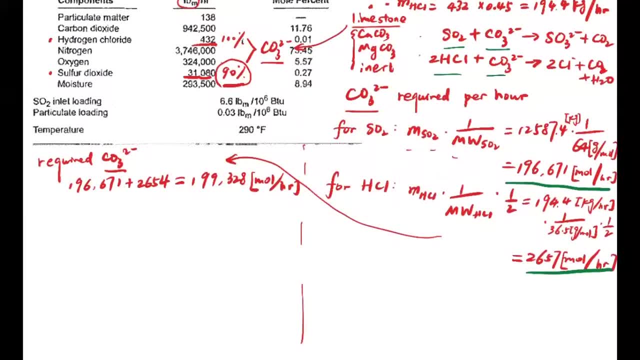 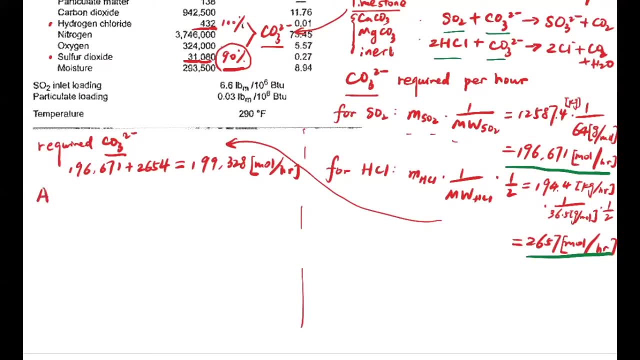 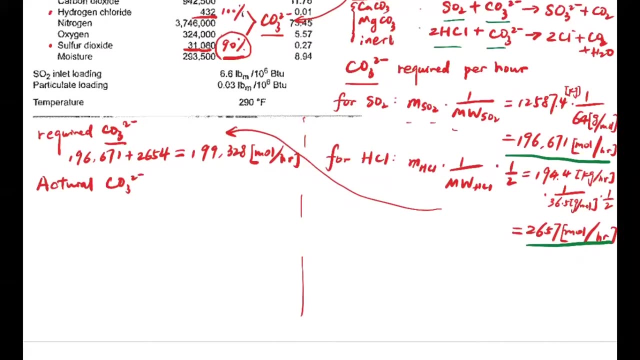 So what that means is we need to provide actual carbon and ions into this calculation. So the actual carbon ions that's needed by this reaction is going to be 199, 328 multiplied by 1.1.. Okay, Okay, so that's going to be 219, 261 mole per hour. 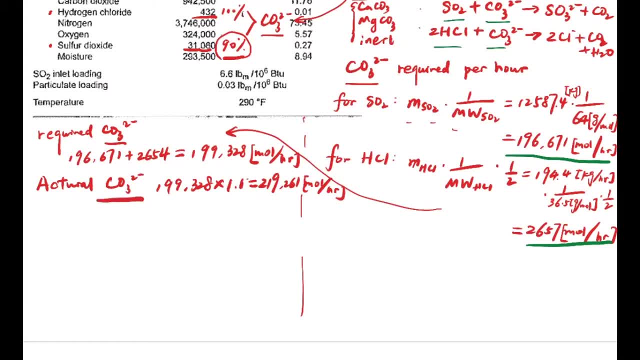 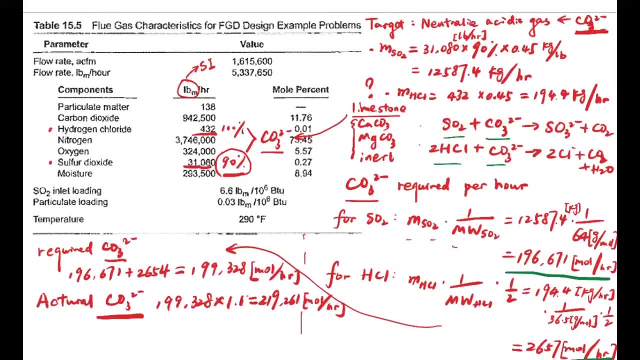 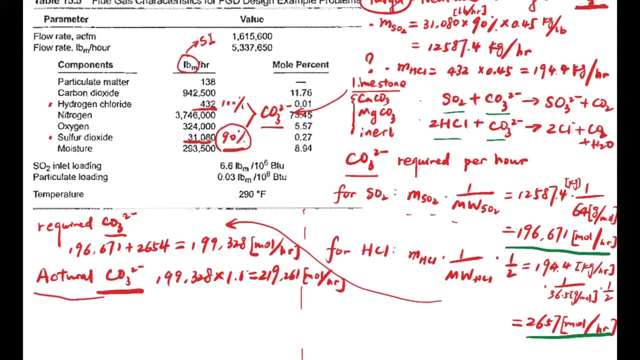 Okay, so this is the actual amount of the carbon ions that's required from this reaction. Okay, So this is our target. What this means is that, in order to react with all of these acidic gases, it requires this amount of carbon. Right, so this is our target. 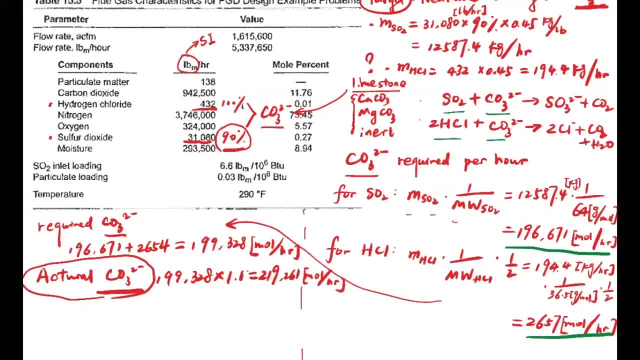 What this means is that, in order to react with all of these acidic gases, it requires this amount of carbon, Right? so this is our target Right? so this is our target Right. so this is our target. So we need to use the carbon ions to go through the reaction, right. 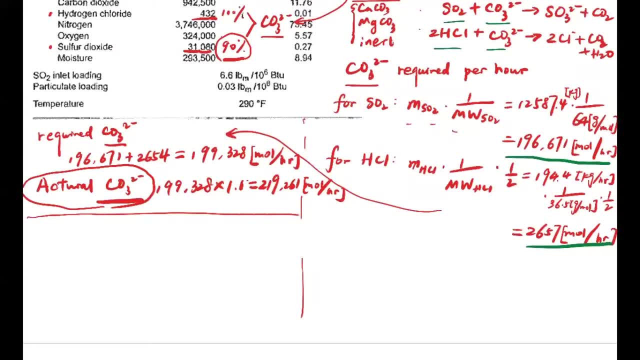 And then what is the reality? Because we need to match the target with the reality, right? So the reality is we're going to use limestone. Let's say that this is our limestone. Okay, So we're going to use the limestone to neutralize, or to use the limestone to provide these carbon ions to neutralize the gas species. 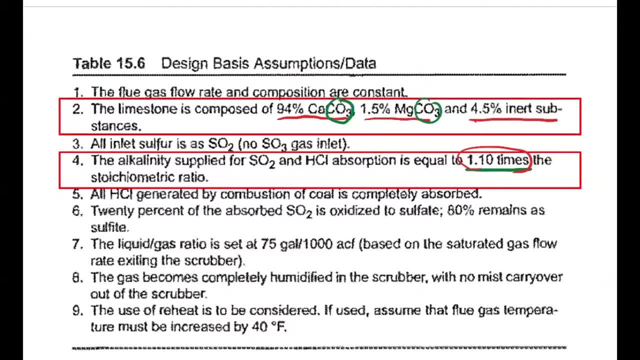 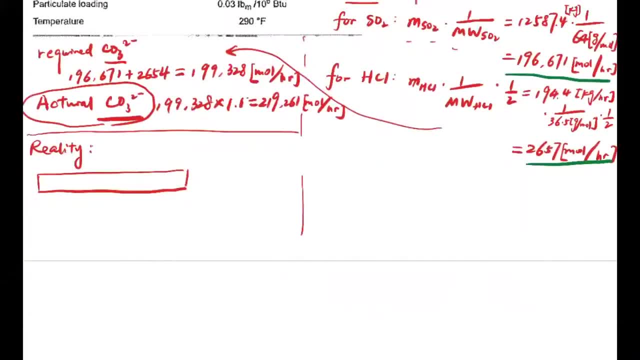 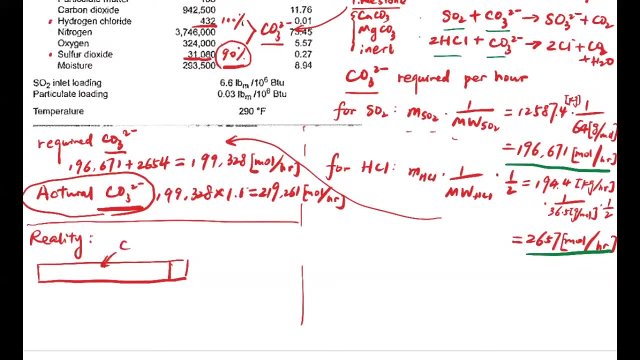 So we mentioned that the limestone is not pure. It contains calcium carbonate, magnesium carbonate and 4.5% of the inert species, right? So we can use this bar to show what that means, right? So let's say, 94% of them are calcium carbonate and 1.5% is magnesium carbonate, and then we have 4.5% of the inert. 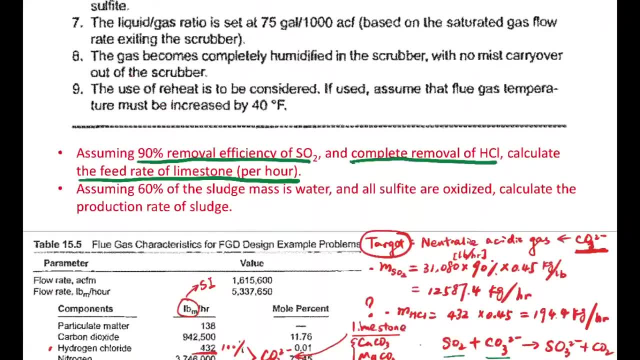 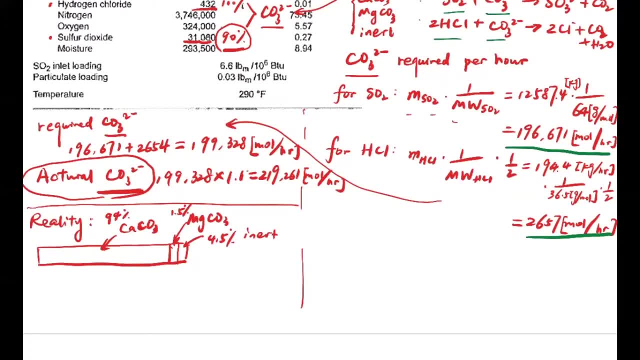 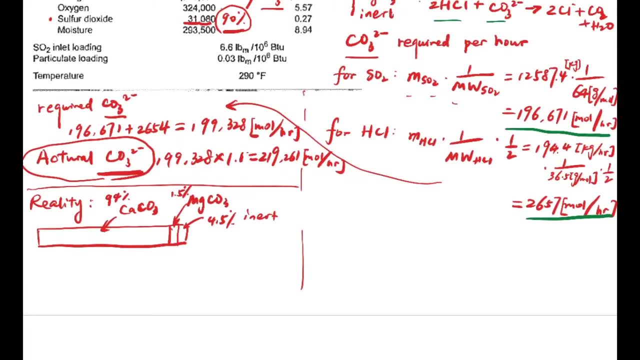 Okay, so we're using this limestone to provide the carbonate ions to neutralize the acidic gas species, And because of that we need to know what is the amount of the carbonate ions it can provide for this standard unit of the limestone right. 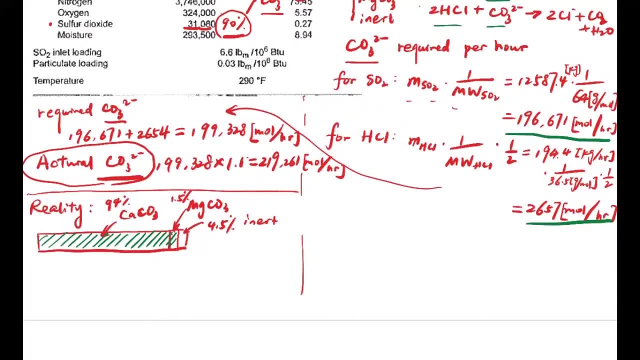 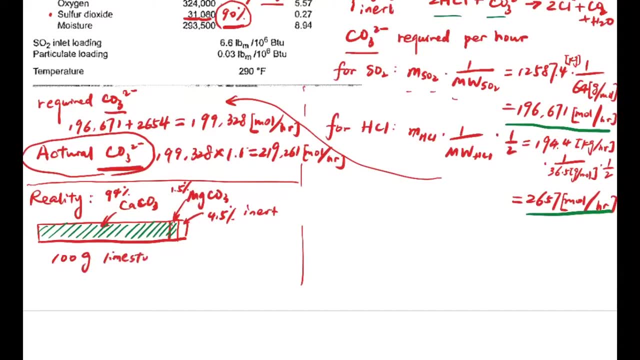 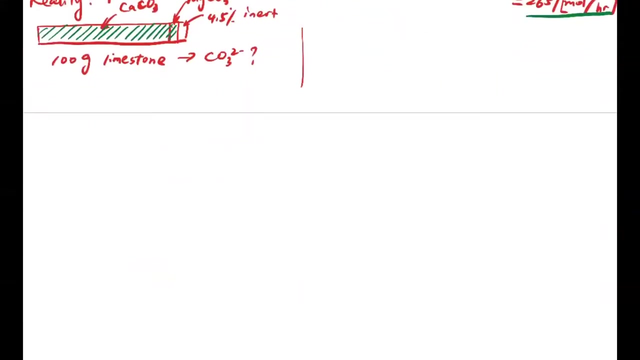 So, For simplicity, what we can do is we can assume that we're trying to analyze 100 grams of the limestone And we need to calculate how much carbonate ions it provides to the reaction, right? So if you assume that there's 100 grams, then what we can directly know is that there are going to be 94 grams of the calcium carbonate. 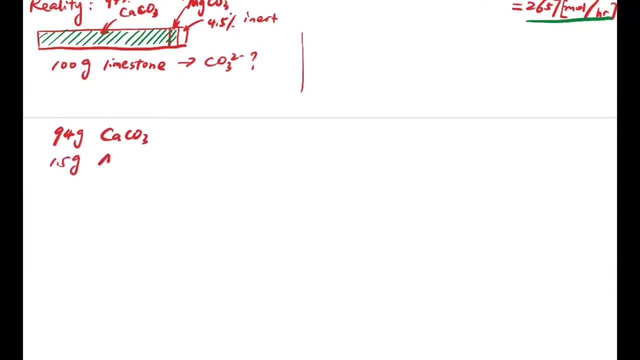 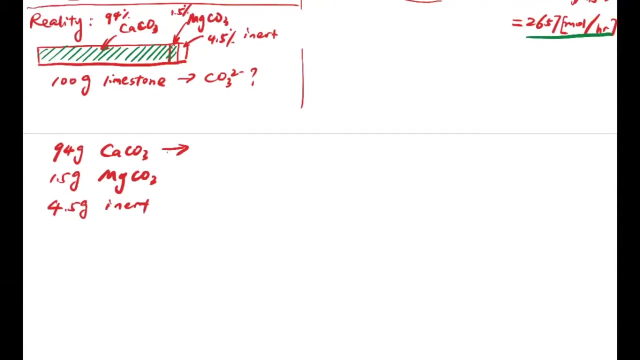 Right, and then 1.5 grams of the magnesium carbonate and then 4.5 grams of the inert. Okay, and if we know the mass of the calcium carbonate, we can calculate what is the moles of the carbonate ions it provides to the reaction, right? 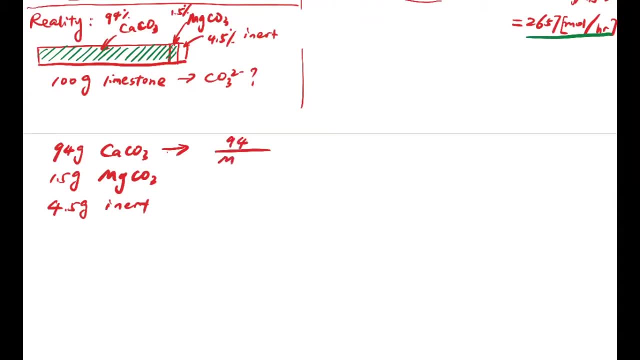 So it's just going to be 94 divided by the molecular weight of the calcium carbonate. Right, so that's going to be 94 divided by 100, which is 0.94 mole of the carbon ions. And in terms of the magnesium carbonate, we'll use 1.5 divided by the molecular weight of the magnesium carbonate, which is 1.5 divided by 84.. 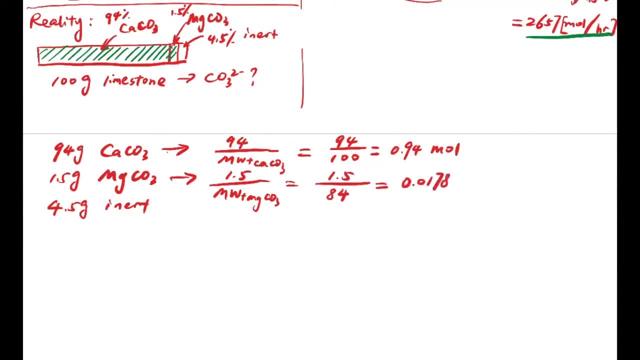 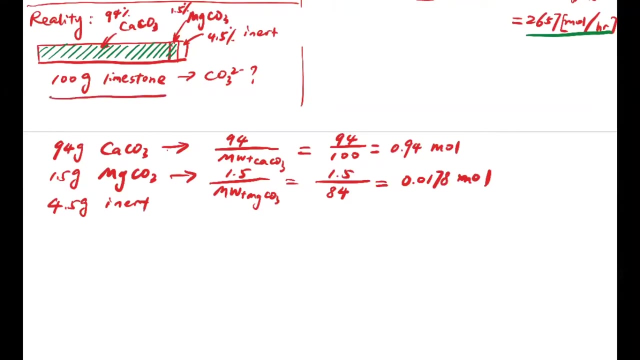 That's going to be 0.01.. Right, So that's going to be 0.078 mole, Okay. so, basically, what we're trying to do is we're trying to analyze 100 grams of the limestone. Within 100 grams of limestone, how many carbonate ions it provides, right? 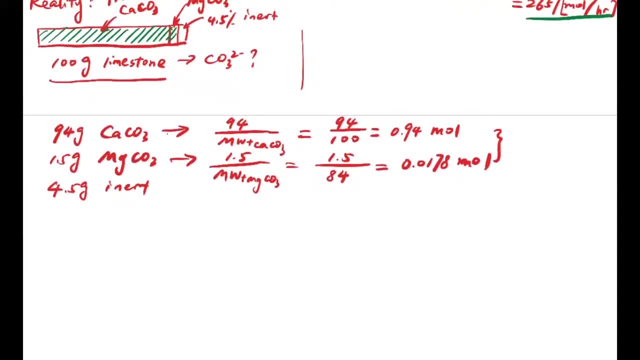 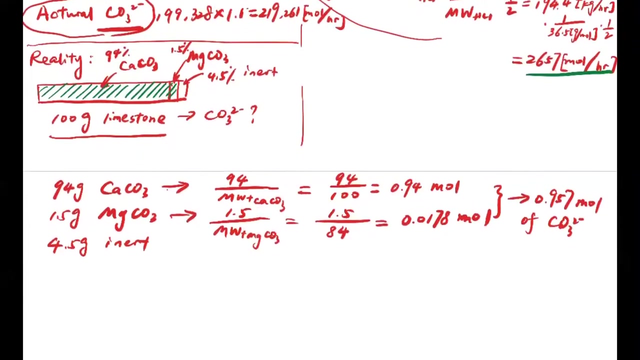 So what this means is that we need to add these up together to calculate the moles of the carbonate ions. right, So that will give us This, gives you 0.957 mole of carbonate ions. Okay, So let's see the problem here. 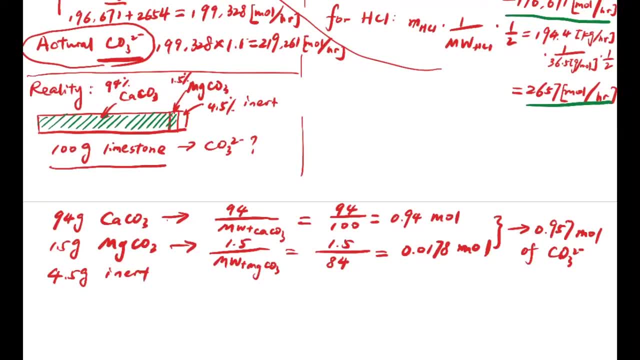 So we know that to neutralize the acidic gases we need this amount of the carbonate ions, And we know that for 100 grams of the limestone we have this amount of the carbonate ions. So for 100 grams of the limestone we have this amount of carbonate ions. 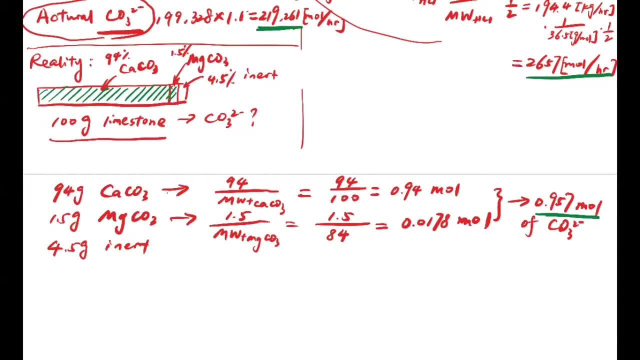 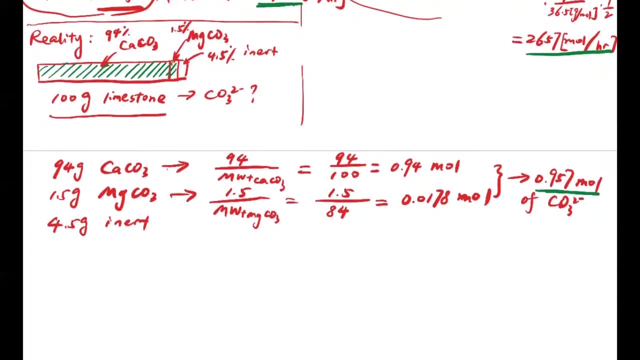 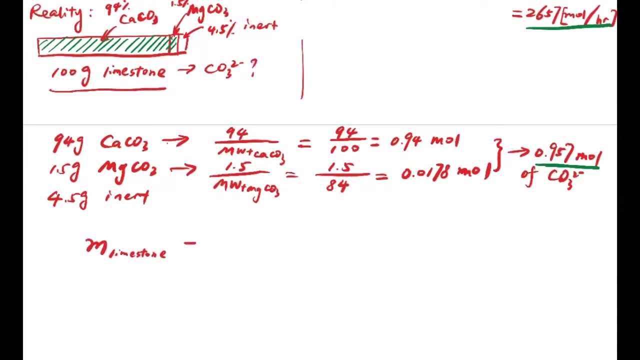 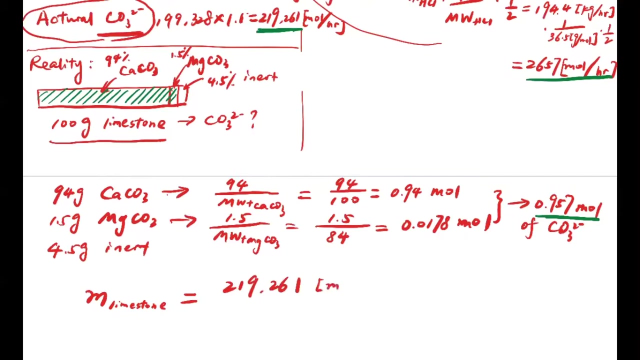 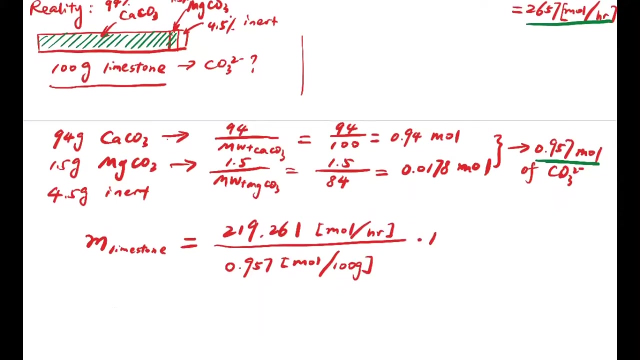 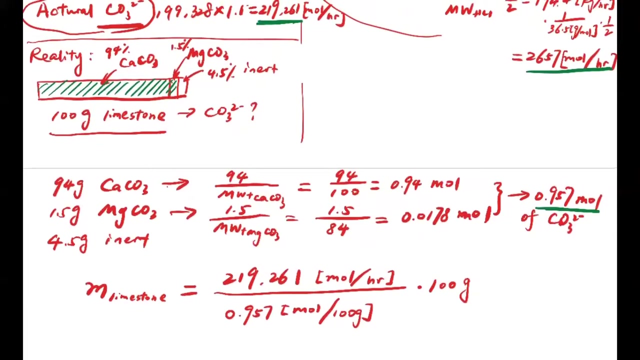 Right, we have this amount of carbon ions and then we can use this relationship to relate to the total required amount of the limestone. right, so that can be calculated by limestone equal to 219261. okay, so what this means is that we'll divide this total required carbon ions by the carbon ions. 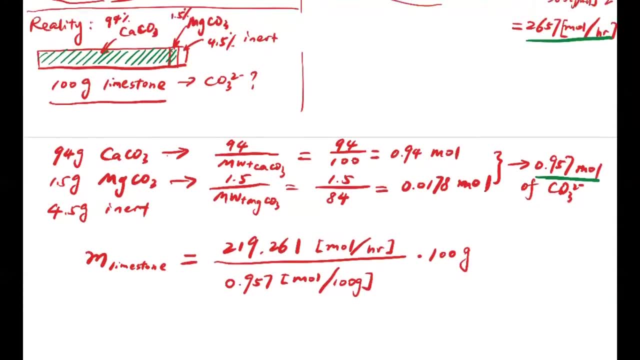 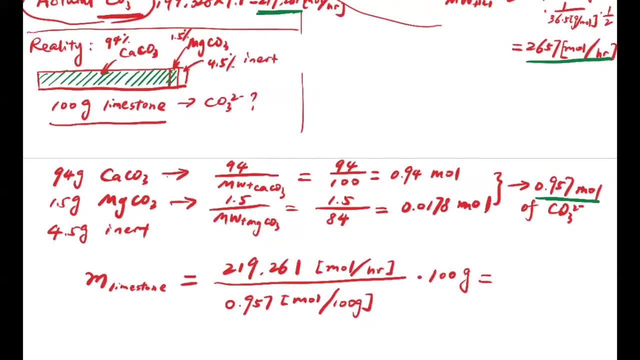 that's provided by 100 grams of the limestone, and then we multiply that by the mass of this limestone, right? so this is going to be the total amount of the limestone we're going to need, and if you use your calculator, you can find out that this is going to. 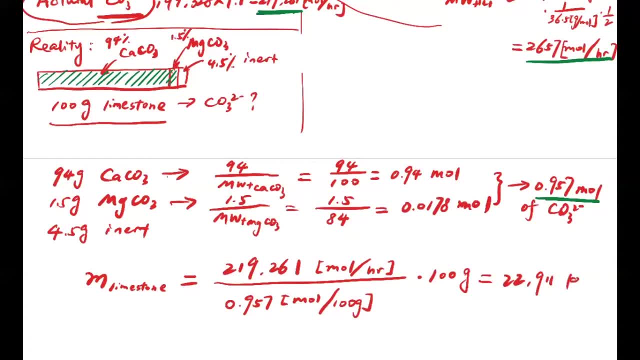 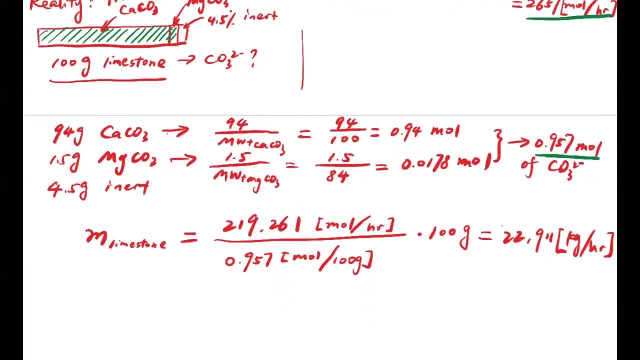 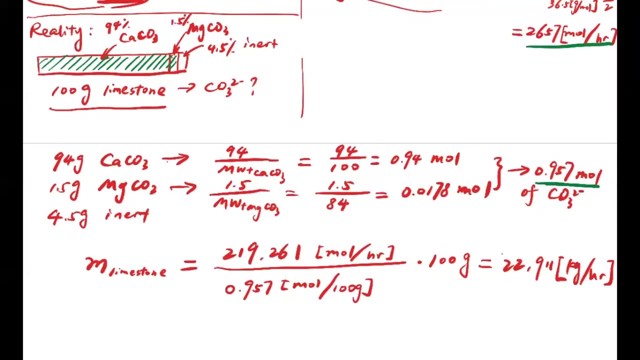 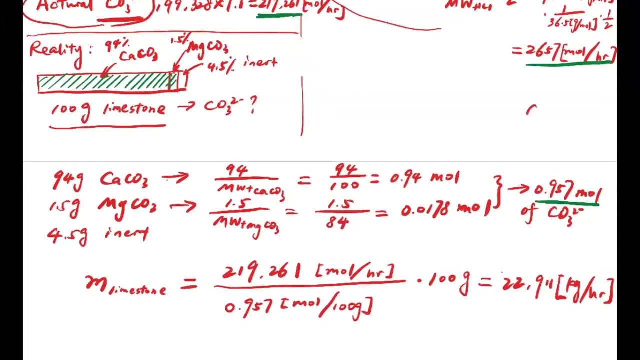 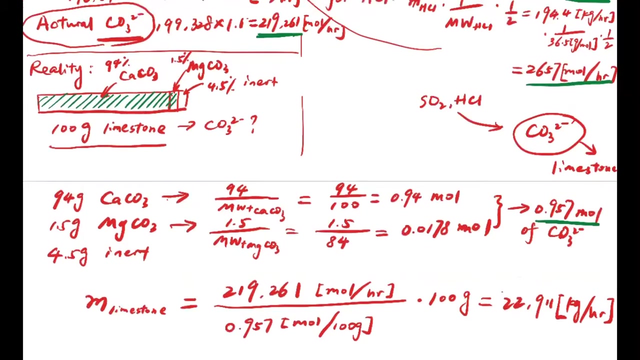 be 22911 kilogram per hour. okay, so i think there are quite many steps of calculations here, but the the general idea is that we're using the carbonate ions as a link between the acidic gases and the limestone. okay, so if we know the generation amount of the acidic gases, then we can calculate. 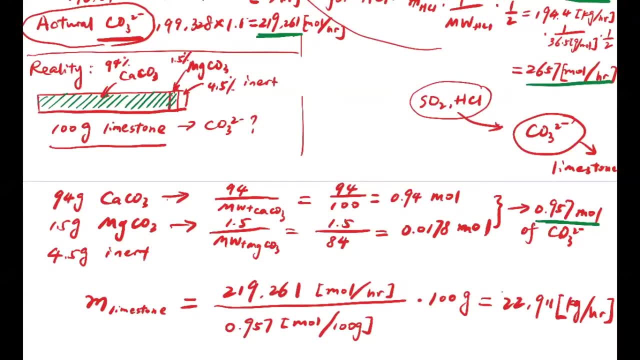 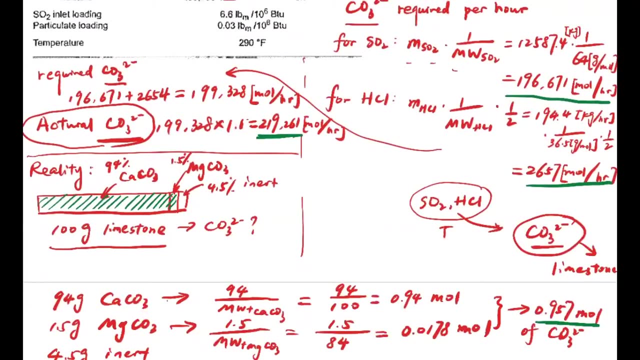 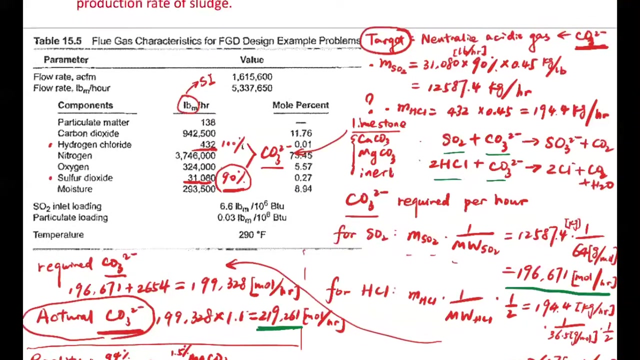 what is for this reaction, and if we know the amount of carbonate ions, then we can, then we can relate this to the amount of limestone that's required for this reaction, right? so that's why we separate this into the target here and then reality in here. okay, so let's just go through this process again. i know that there are quite many calculations. 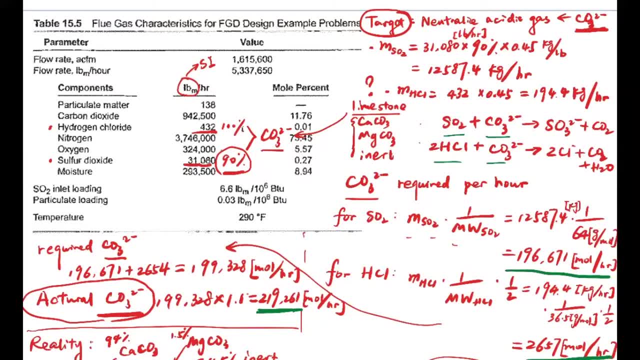 here. i think you also have a homework problems, homework problems on this, similar, similar type of questions. i think you'll get more practice in here. i admit that that this is indeed quite complex, but the general idea is that we're trying to use the carbon ions as a bridge to calculate. 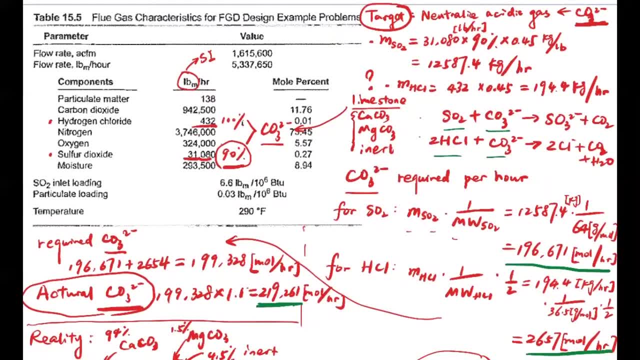 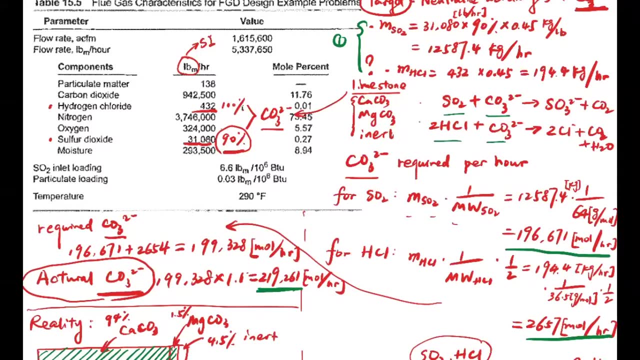 this process. okay, so we can separate that into multiple steps. so the first step is to find out how much acidic gas we need to deal with. okay, so that's generally given by the table or by the question there, right? similarly, we can calculate what is the amount of sulfur dioxide we can generate from the coal. 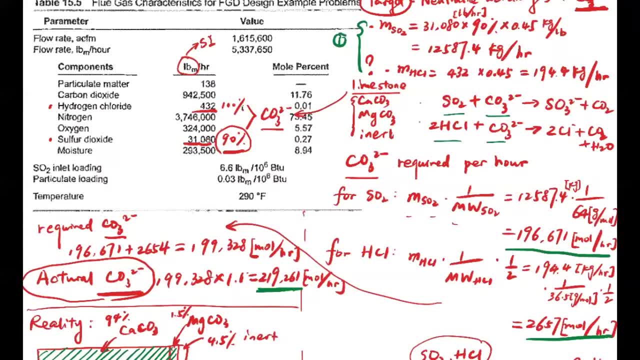 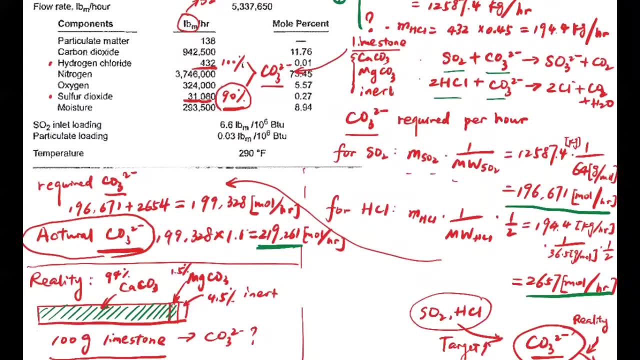 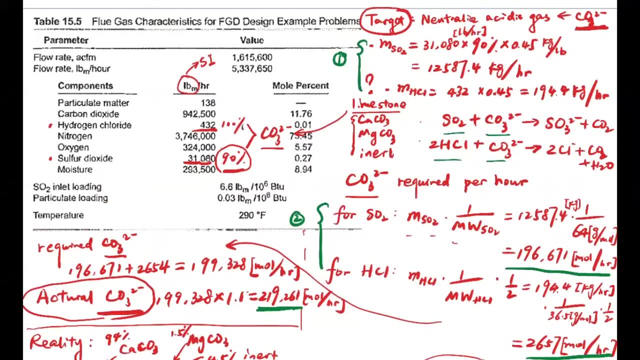 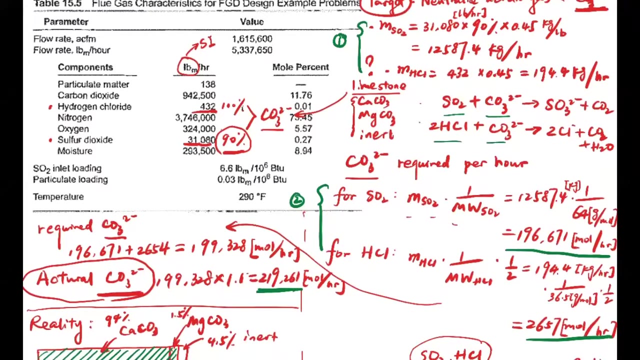 fire power plant. so that's already known, right? so the first step is try to see how much of the acidic gas we're trying to deal with, right? and the second step is convert the acidic gas amount into the carbon ions. it requires to react. because if we know the amount of sulfur dioxide, we should be 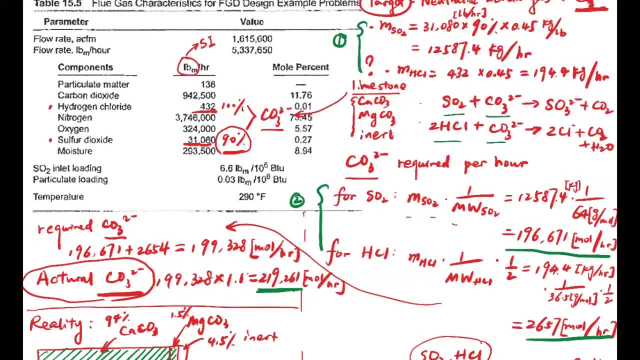 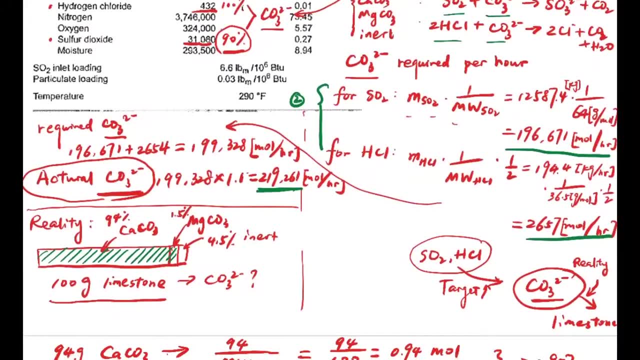 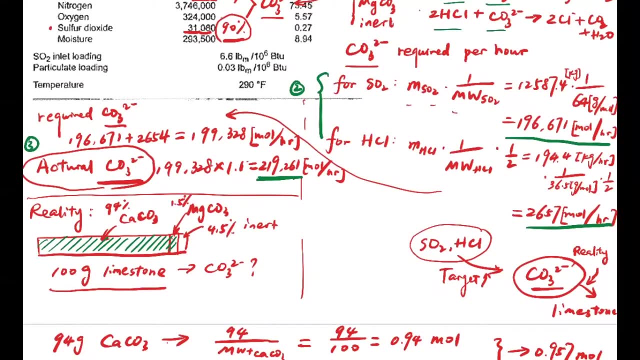 able to know how many carbon ions it reacts- right, because it reacts at one to one ratio there. and the third step is to calculate what is the actual carbon ions it requires, right? we mentioned that it's going to react at a 10 percent more of the limestone, right? so that's why we multiply that by 1.1, basically to add this extra limestone. 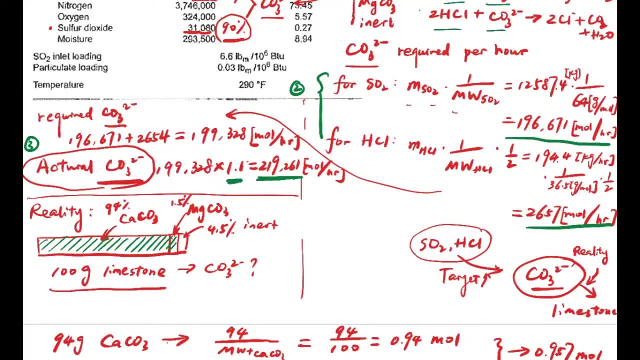 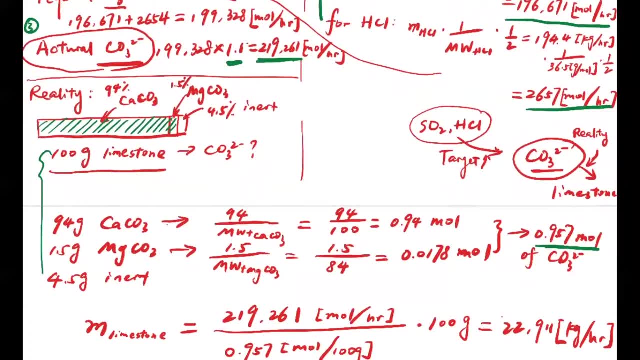 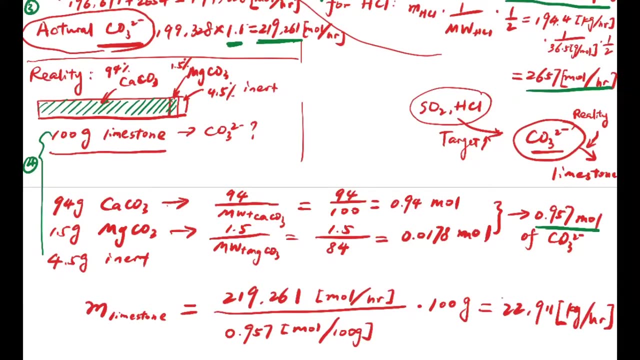 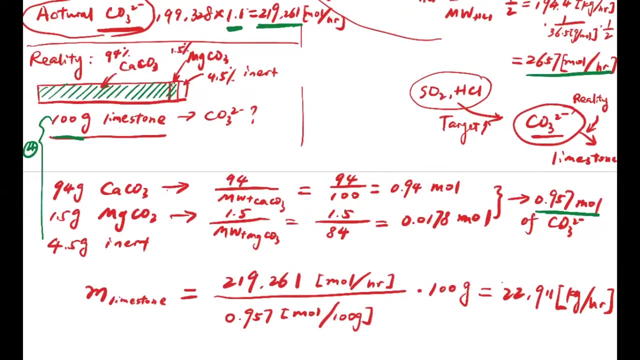 and this is the actual carbon ions it requires to neutralize the city gas. okay, and the fourth step is to find out how many carbon ions can be provided by the limestone. here we're using an example of the limestone. we can calculate what is the weight of the calcium carbonate. 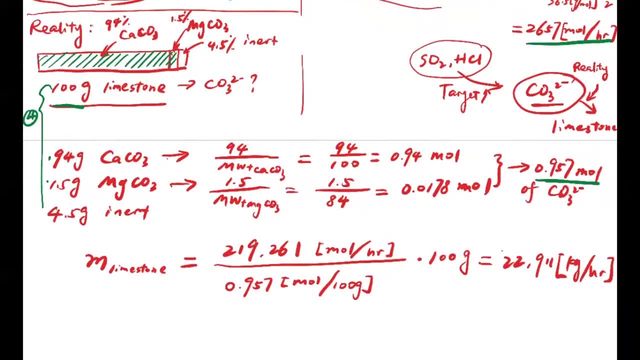 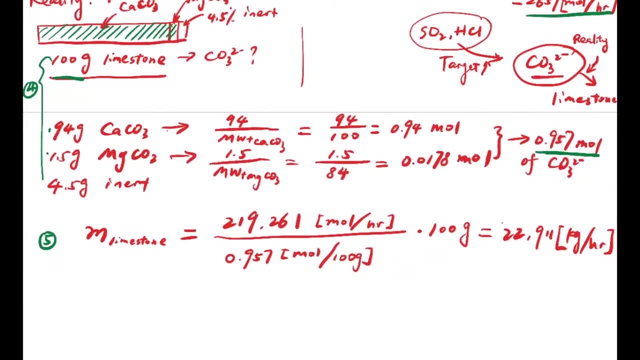 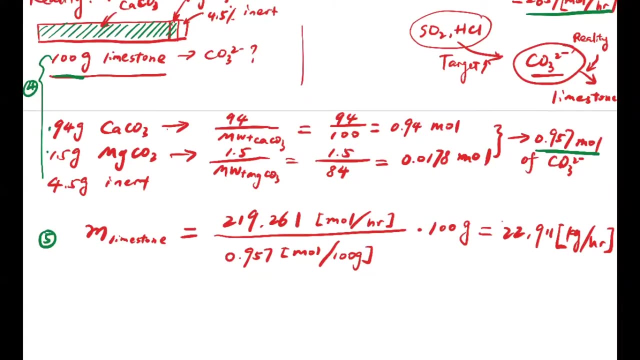 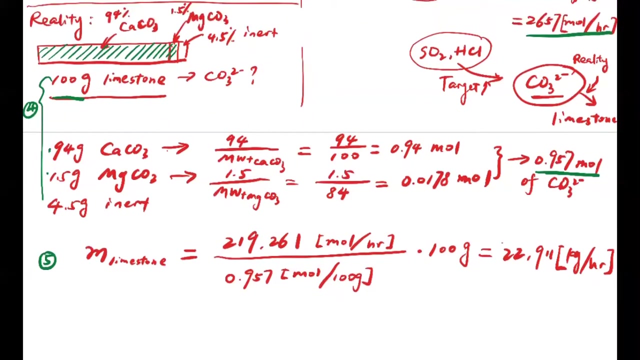 what is the weight of the magnesium carbonate and then calculate the carbonate ions. right and finally, the fifth step is to relate this carbon ions amount and then calculate what is the total mass of the limestone. okay, so this is where we calculate the feed rate of the limestone. 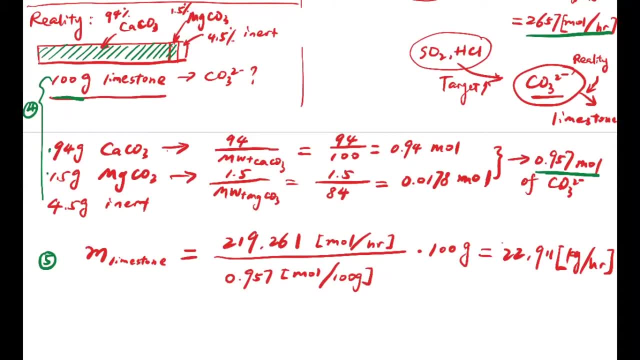 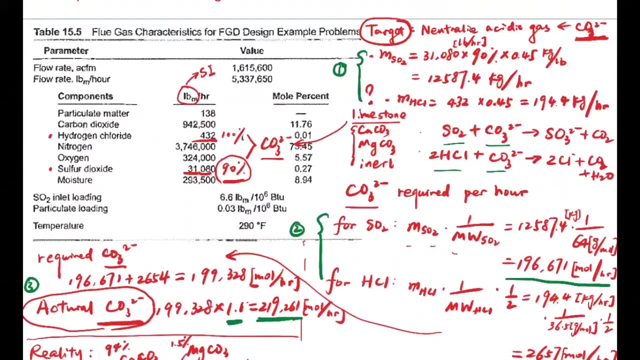 so everything is based on the starry geometric ratio and i would say that you're going to use the same method for your trisorbid injection. let's say we're introducing trona into the system or introducing lime into the system, right? we know that the lime 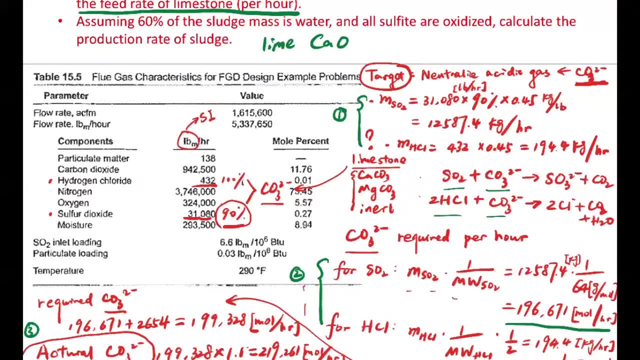 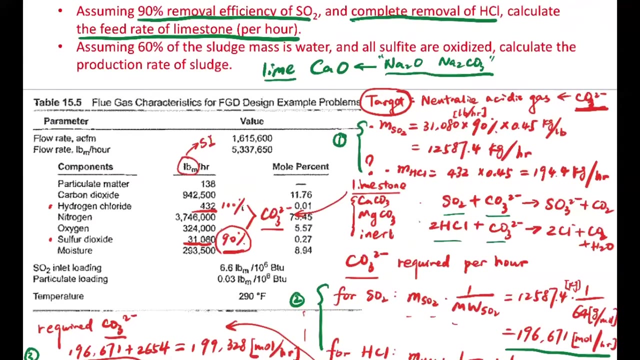 is not pure um calcium oxide right. so there's always some other chemical species, for example um sodium oxide right or sodium carbonate. so you need to find out what is the chemical composition of the lime right. and basically the lime will react with the um, with the acidic gases, similar to the ratios. 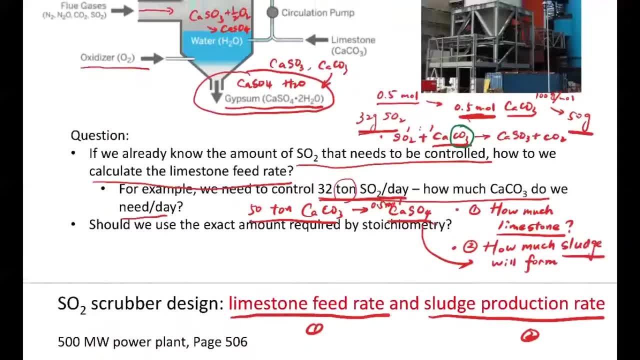 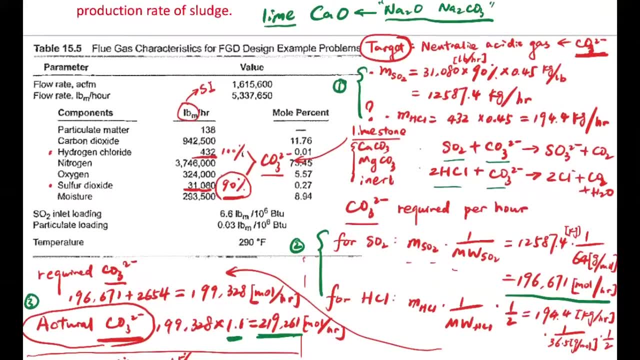 that are provided here, right? for example, i think we also have the reactions here, okay, so basically it's reacting with the oxygen negative ions, right? or you can think of that as the hydroxide ions. okay, so based on these reactions, we can find out what is the required. 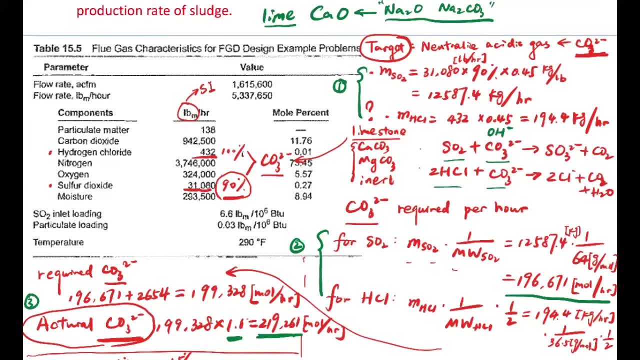 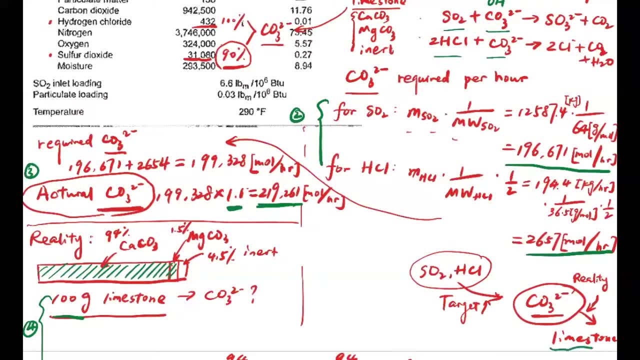 oxygen ions or what is the required hydroxide ions, and use that as a bridge to relate the amount of the acidic gases and the actual required amount of your either lime or trona into the system. right, so this is how we solve the feed rate of the limestone. we mentioned that. 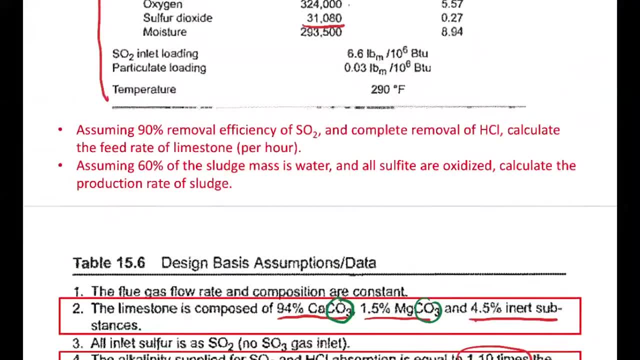 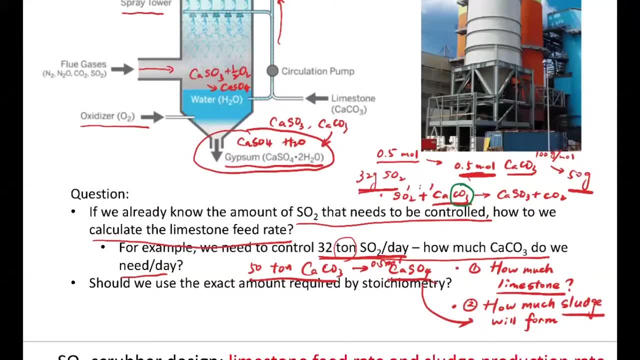 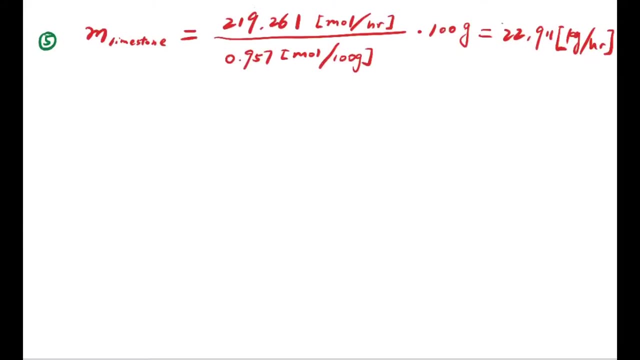 for the design problem. we're also interested in: what is the sludge production rate? okay, so the sludge is just the react, the, the product that's coming out of this reaction. right, so we mentioned that. if we consider the product, so that's going to form calcium sulfite first. 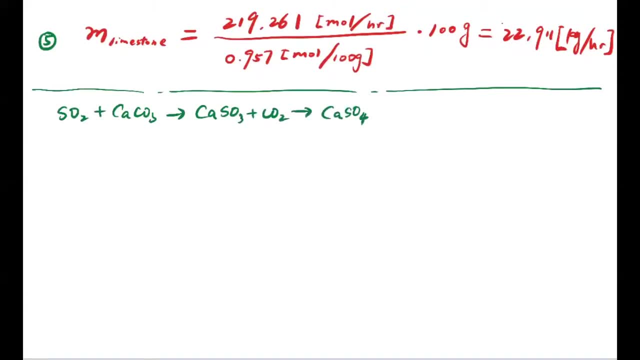 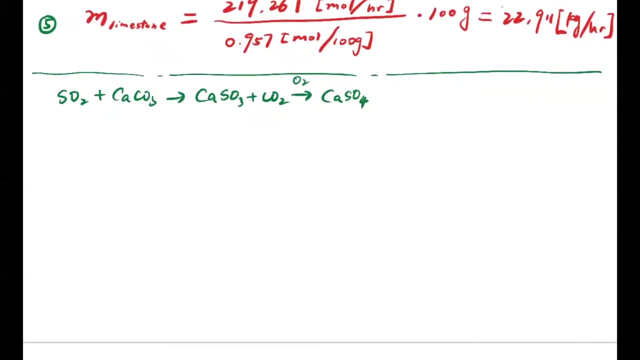 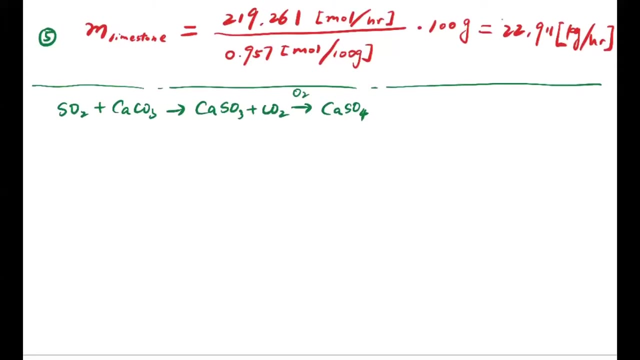 and then, finally, we're going to form calcium sulfate, mainly because we add oxygen into the system. right, we oxidize these, uh, calcium sulfide, and you see that in this problem, we're basically providing more limestone into the scrubber and because of that, the sludge is also not going to be a pure substance. 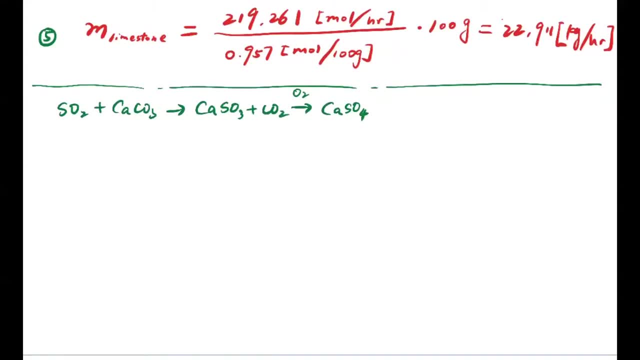 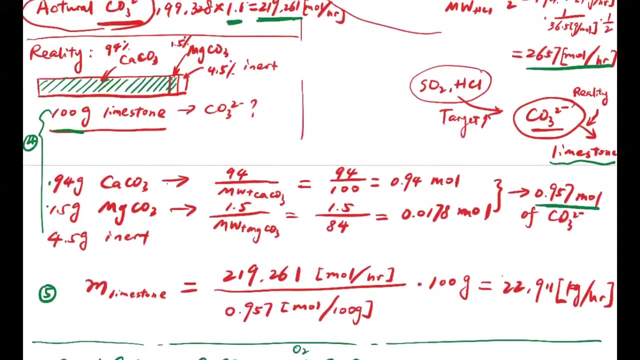 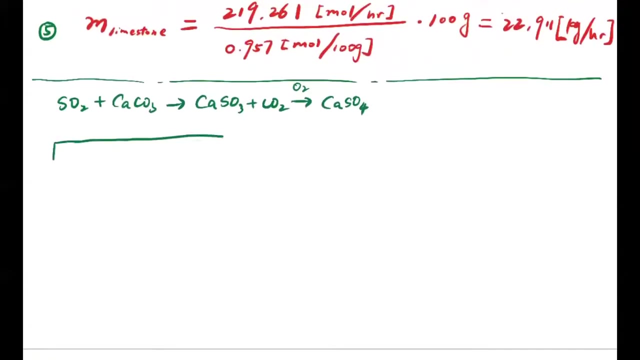 right, we need to consider that there are um. they're also inert in the system, right? so what we can do is we can also draw a bar that's similar to this limestone bar here. so let's say that we're trying to gen, we're trying to analyze 100 grams of the sludge. 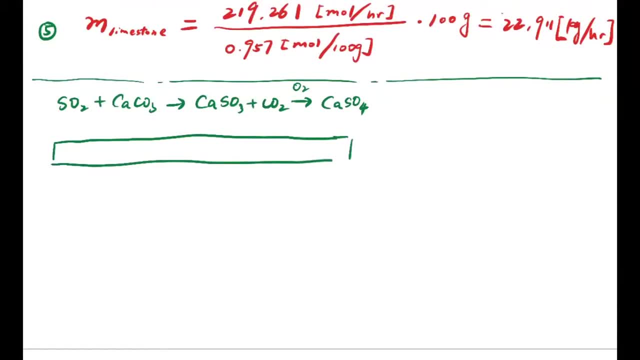 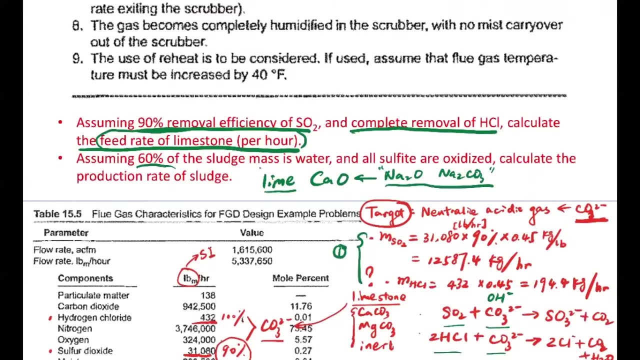 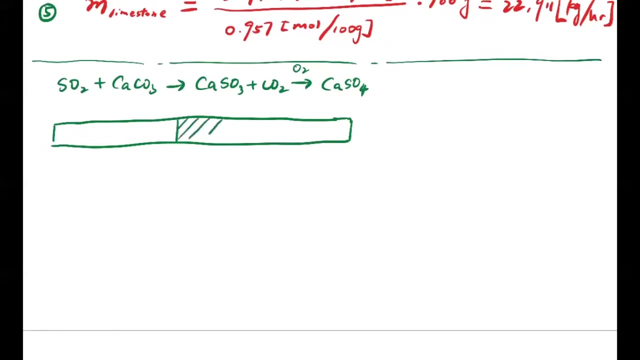 or the, the product coming out of the scrubber. so you see, for this question, it assumes that 60 percent of the mass is water, right? so from this bar here we know that actually 60 percent. we don't need to consider that. so that's going to be just pure water, okay. 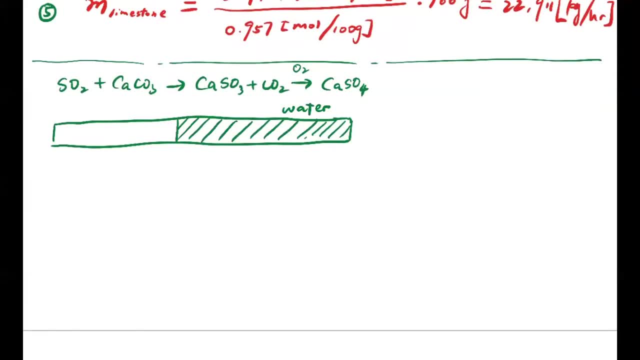 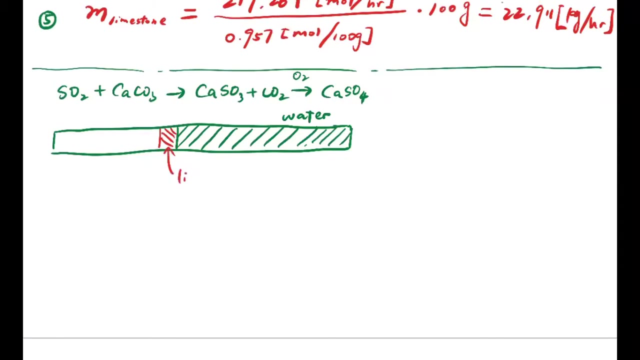 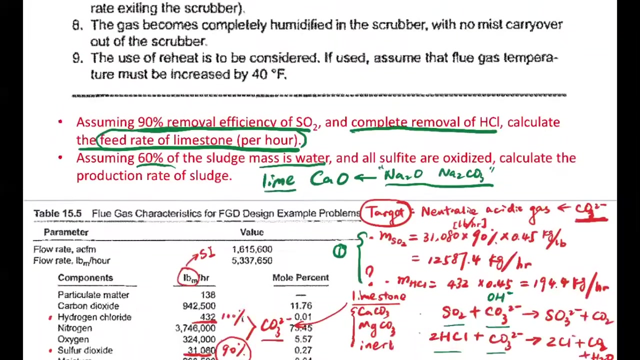 and the remaining 40 percent are going to be the solid okay and further. if we consider the solid composition, it's actually made of quite many things. so first we have a proportion of the limestone that's that are not being reacted. so remember, in this problem we assume that we provide 1.1 times of the amount that's required. 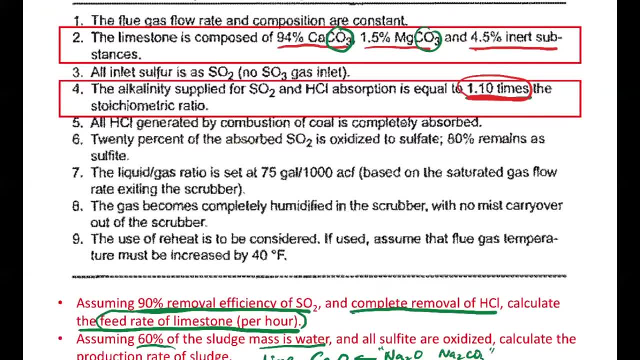 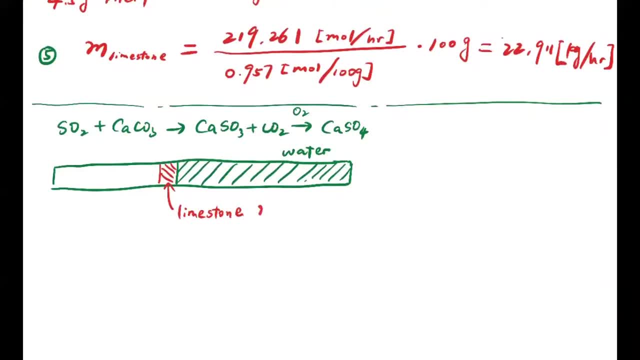 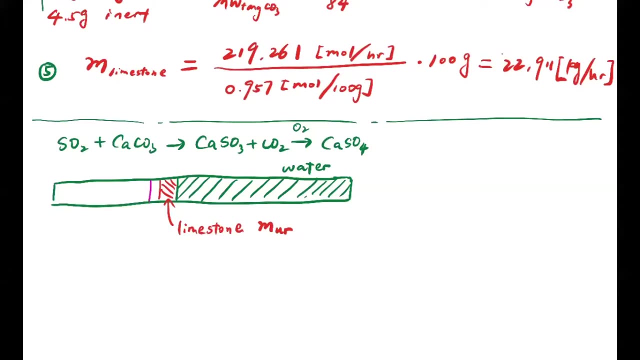 by the stoichiometric ratio, right, so that 10 percent extra are not being reacted. so we can say that this amount, this amount, is unreacted, okay. and then for the reacted limestone, we know that there is further a fraction that's inert, right, and then we have a fraction. 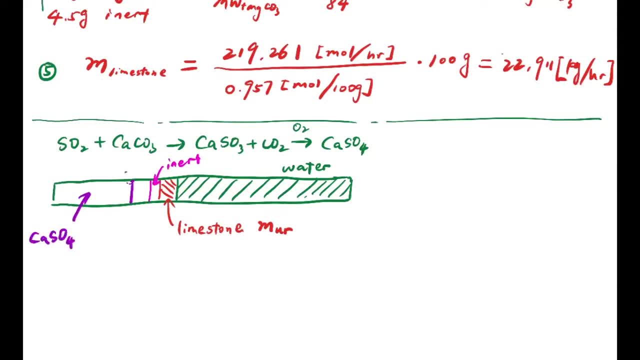 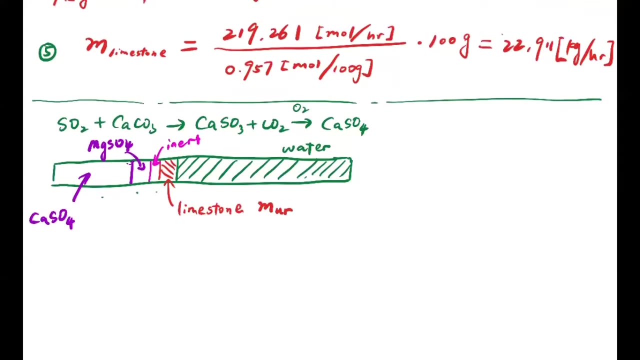 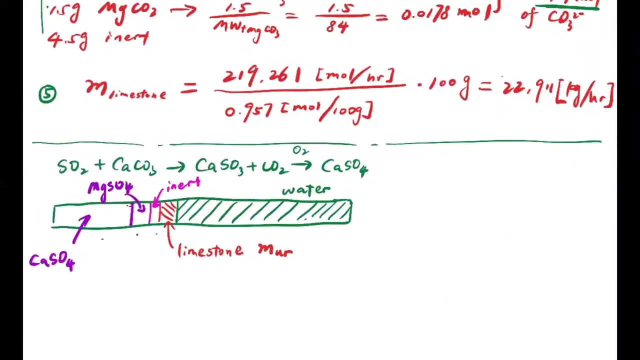 that's calcium sulfate, and then we have a fraction of magnesium sulfate. okay, so to calculate what is the total amount of the sludge, we need to analyze basically piece by piece and add them all together. right? so for this problem, let's also basically try to solve it, or target at it one by one. okay, from the previous problem we 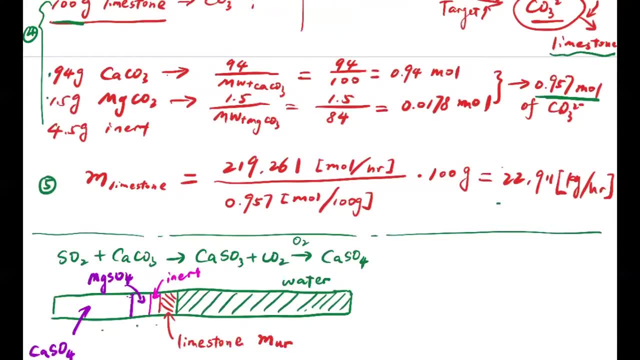 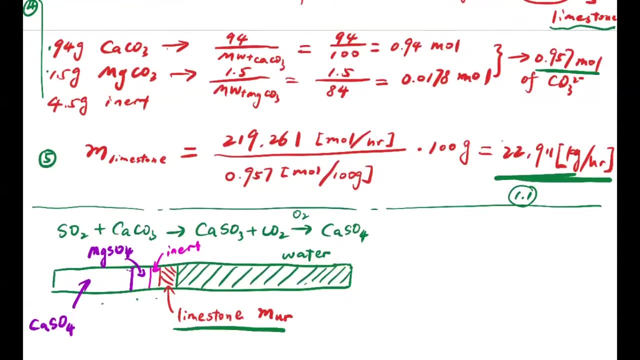 know that the total amount of limestone is going to have this value here and we know that it's basically 1.1 times of the amount that's required by the stoichiometry, so we can first calculate what is the unreacted limestone. okay, so the unreacted limestone is going to be two, two, nine, one one. 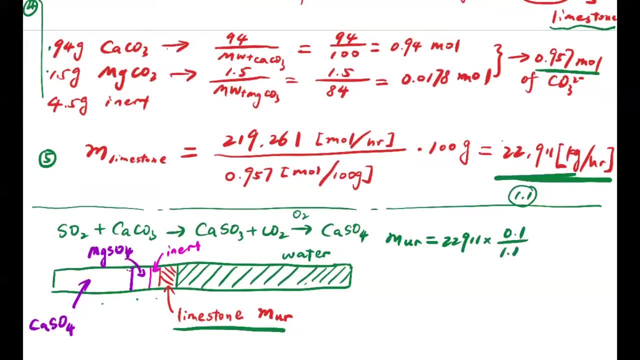 multiplied by 0.1, divided by 1.1. okay, so we mentioned that among this 1.1 total amount of the limestone, basically one is being reacted from this process and 0.1 is just extra right. so this is going to be the unreacted fraction of the limestone and you can find out that this amount is: 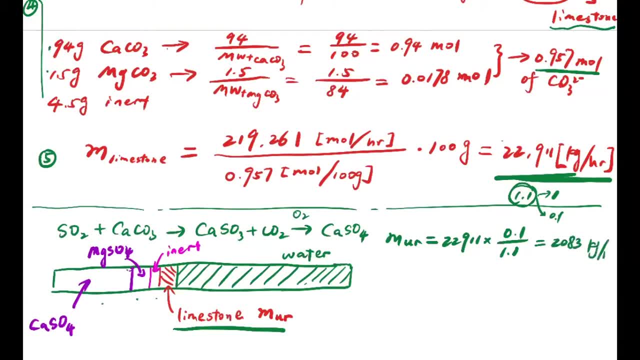 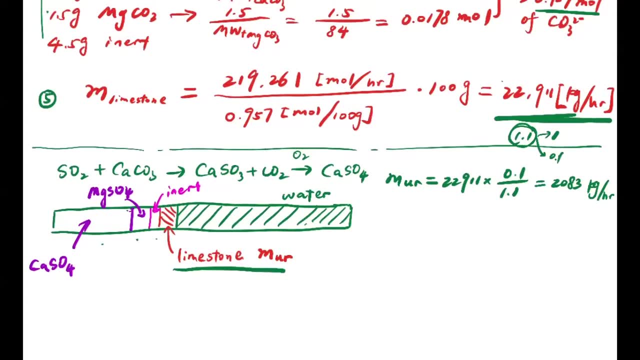 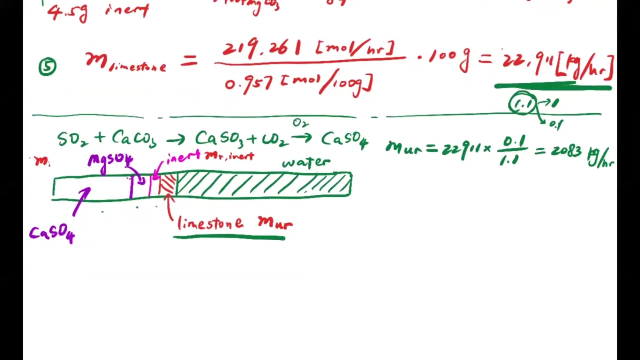 2083 kilogram per hour. okay, this is the, and you are, and we should also write out these- and reacted inert, and this is for the magnesium sulfate that's going to be. and reacted magnesium sulfate, and here we have m reacted calcium sulfate. okay, so the total amount should be all of these. 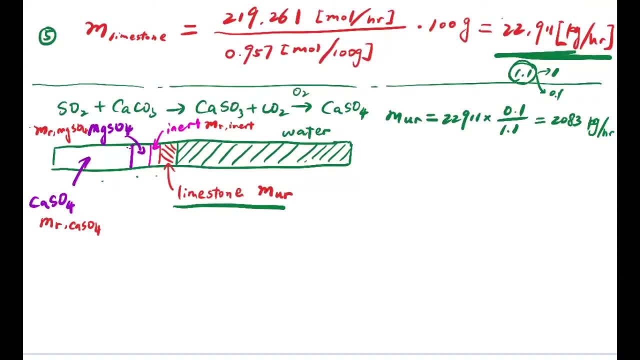 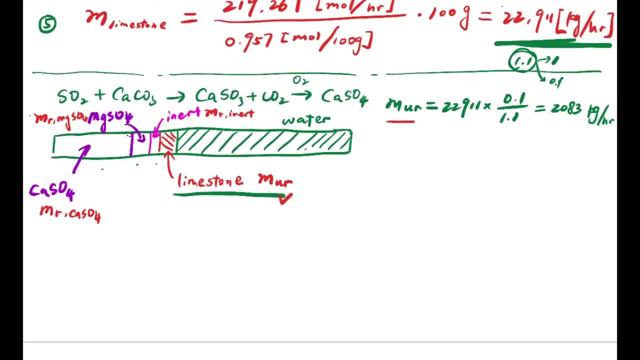 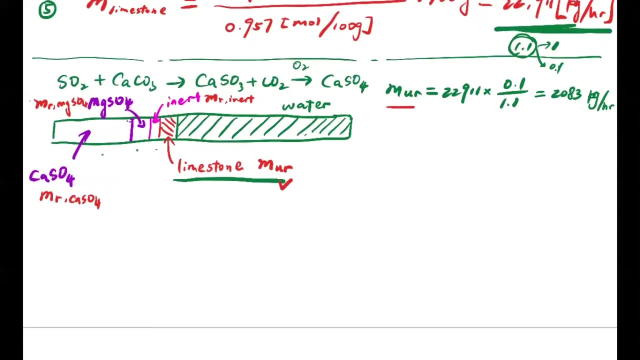 added together plus the water. okay, so that's, that's going to be the production rate of the sludge. so we first calculated what is the unreacted limestone here, right? so if we can calculate what is the area unreacted limestone, we can also calculate what is the reactive limestone. so we can use a similar method. 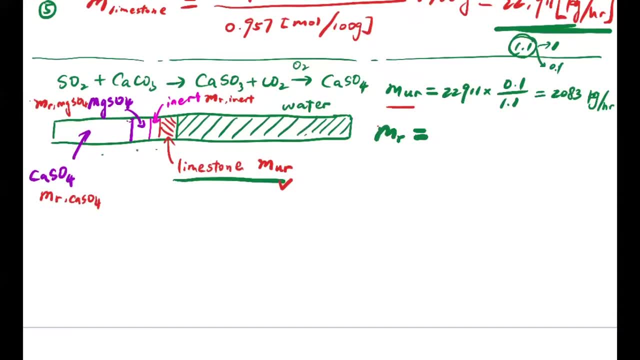 okay, so we can use a similar method and then just multiply this two to nine, one one- and then multiply by one, divide by 1.1. okay, so this is a reacted amount of the limestone, and that's going to be 20828 kilogram. okay, so this is the reactive amount of the limestone, and that's going to be 20828 kilogram. 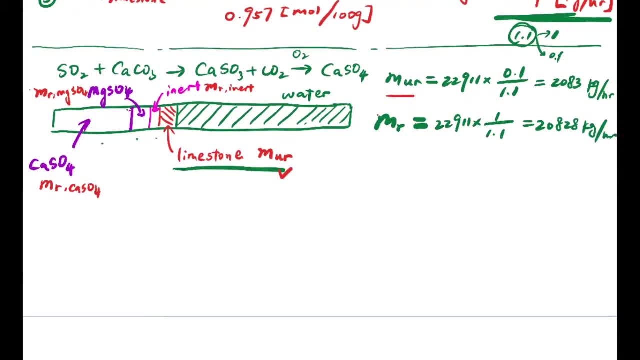 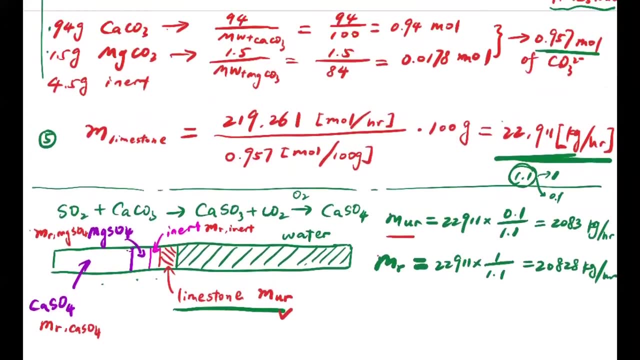 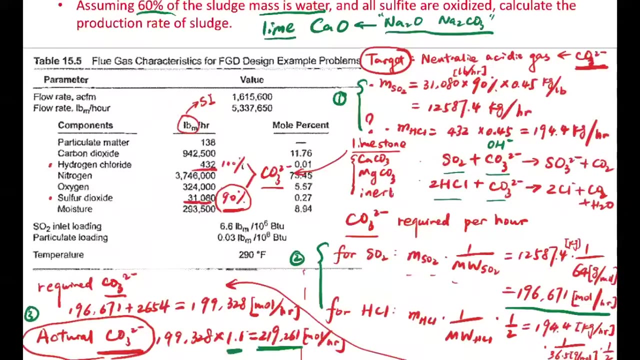 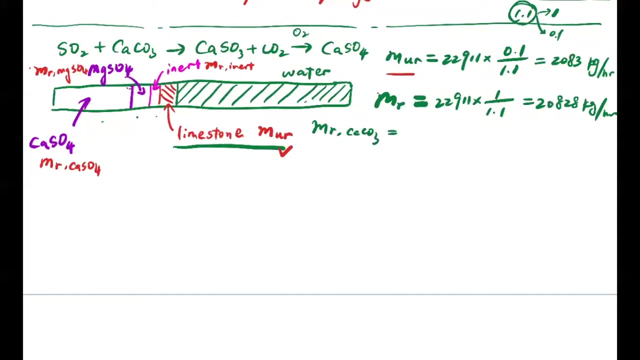 kilogram per hour. all right, and then if we know the react, the reacted limestone, then based on the assumption that 94 percent of them is calcium carbonate, 1.5 percent is magnesium carbonate, then we can calculate what is the reacted amount of calcium carbonate. so that's going to be two zero nine two. 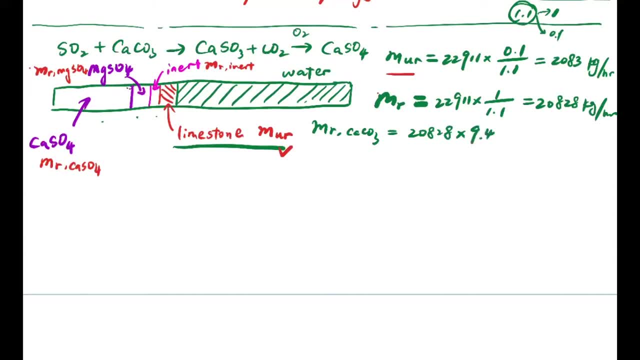 eight to eight, okay, multiplied by ninety four percent. similarly, we can calculate what is the reacted amount of magnet magnesium carbonate and also the inert: okay. so in terms of the inert, its composition is not being changed, right, so it's just going to be the amount that's going to fill. 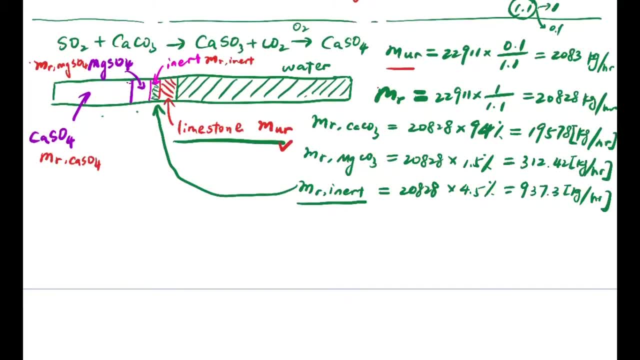 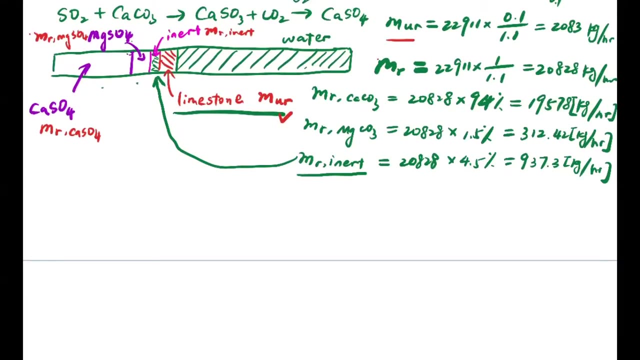 in this pie here. okay, in terms of the calcium carbonate and magnesium carbonate, their composition changed, so their composition changed to magnesium sulfate and calcium sulfate, right, and since we already know the mass of them, then we can convert them first into the, the rate in in moles, and then 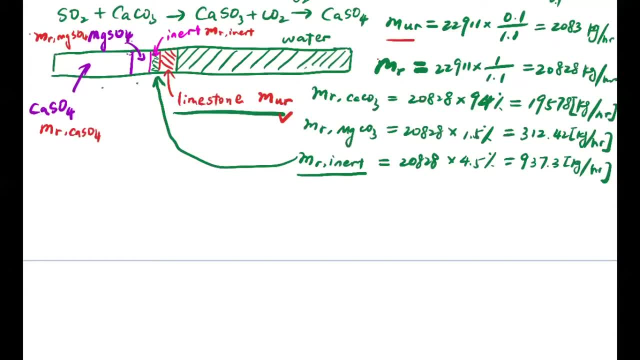 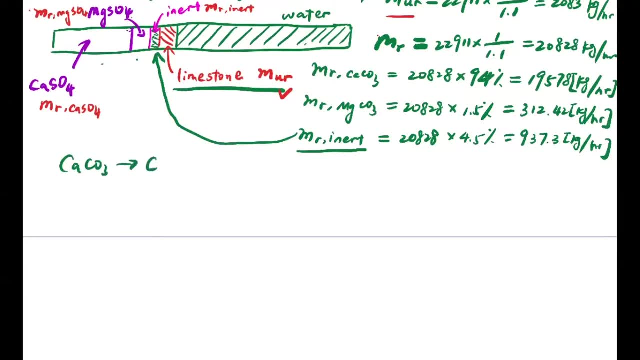 further convert the rating moles into the mass right. so we know that calcium carbonate get converted into the calcium sulfate. because of that, the production rate of the calcium sulfate is going to be the mass flow rate of the calcium carbonate divided by its molecular weight and multiplied. 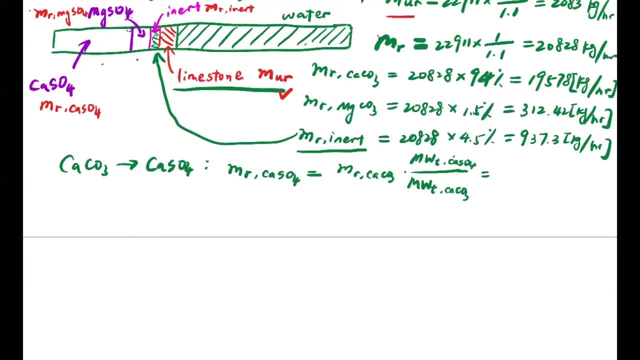 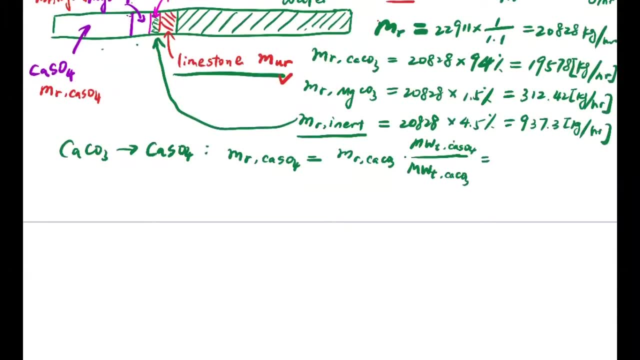 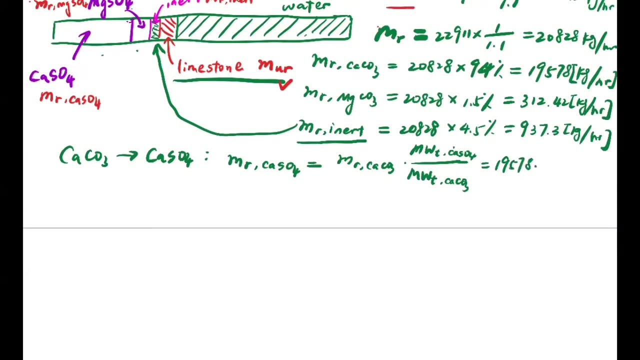 by the molecular weight of the calcium sulfate. so that's going to be one, nine, five, seven, eight, 36 divided by 100. okay, so you can get the mass flow rate of the calcium carbonate. so that's going to be the mass flow rate of the calcium carbonate. 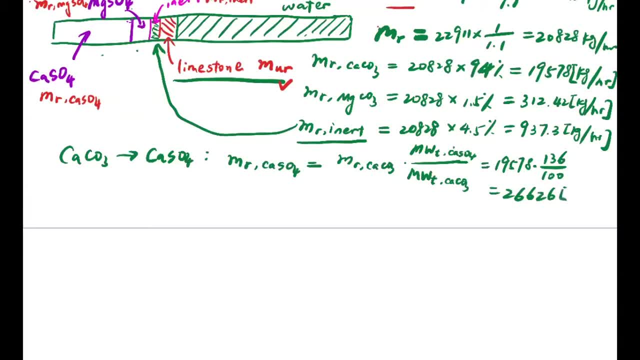 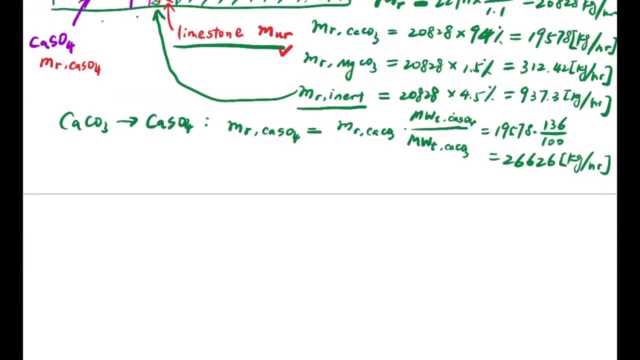 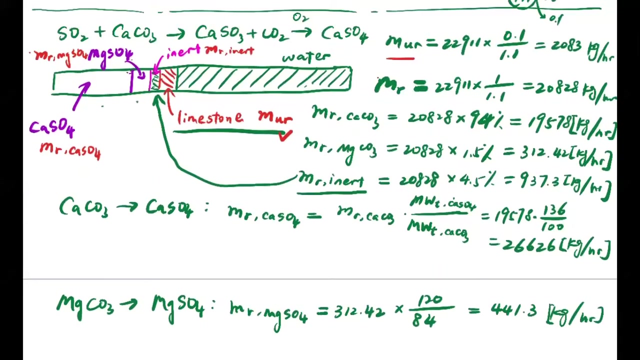 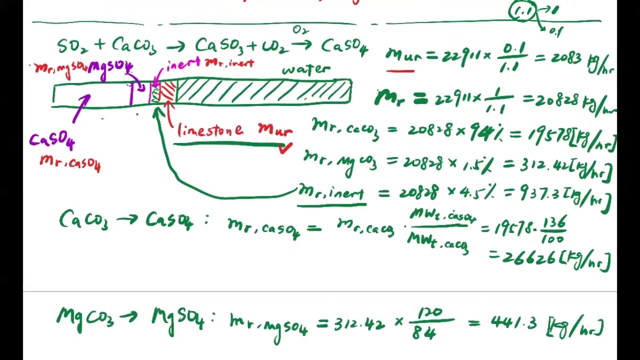 two, six, six, two, six kilogram per hour. okay, we can do the same for the magnesium sulfate. okay, so now we have. we have calculated all the terms that's required for this sludge. okay, so now we have. we have calculated all the terms that's required for this sludge. okay, so we have. 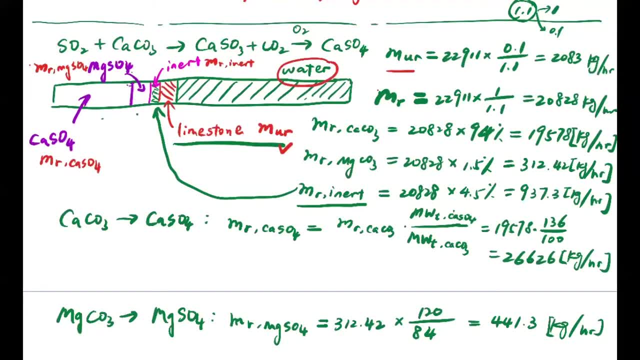 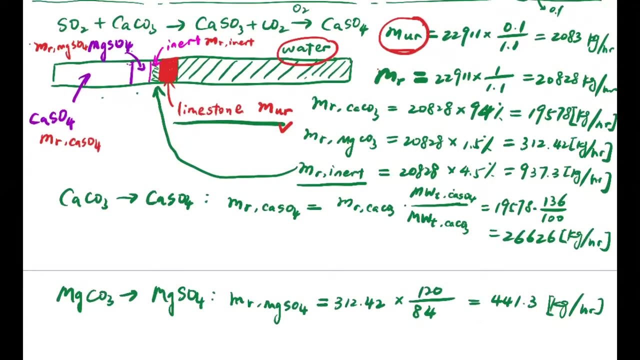 first we know what is the water right and then we calculate what is the unreacted amount of the limestone and that's basically the pie chart here. so this is the extra amount of limestone we provide to the scrubber right, and then we were able to calculate what is the inert, that's in the reacted limestone. 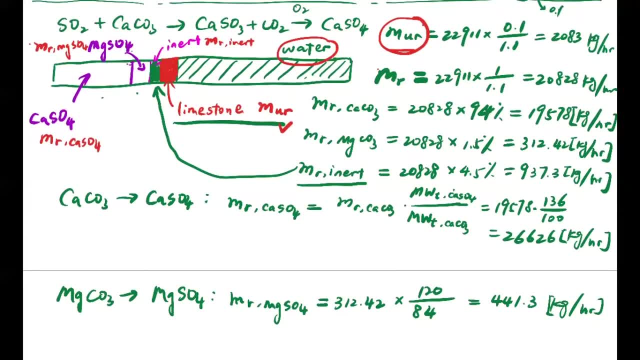 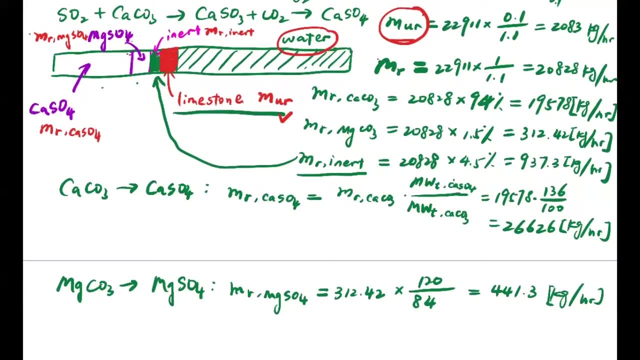 so that is this amount here, okay. and then in the reactive limestone, we were able to calculate what is the, the formation rate of the calcium sulfate- right, the calcium sulfate is here, okay. so finally, we have the magnesium sulfate, which is here, okay. and these are calculated based on the reacted amount of the limestone here, okay. 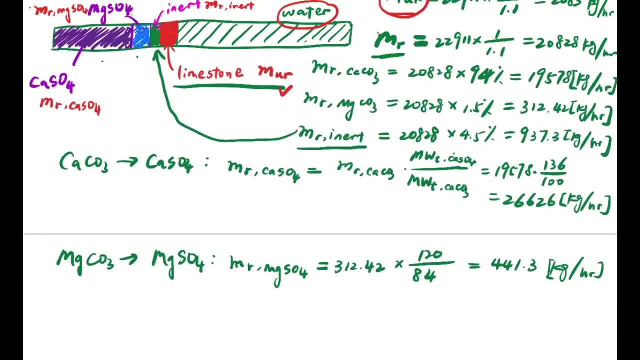 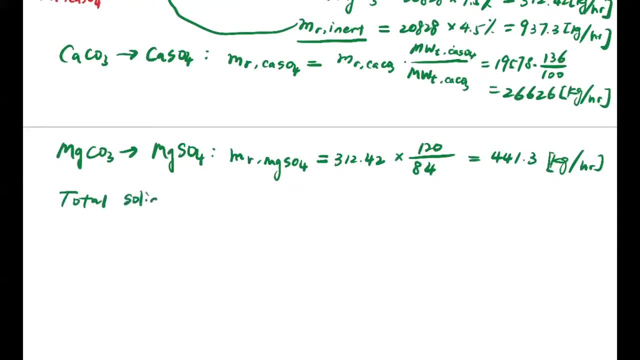 so now we can just add everything together. so first we can calculate what is the total solid in the sludge. so that is going to be the unreacted limestone plus the reacted limestone and the inert inside. okay, so now we can just add everything together and then the reactive limestone, magnesium sulfate, and the reactive limestone calcium sulfate. 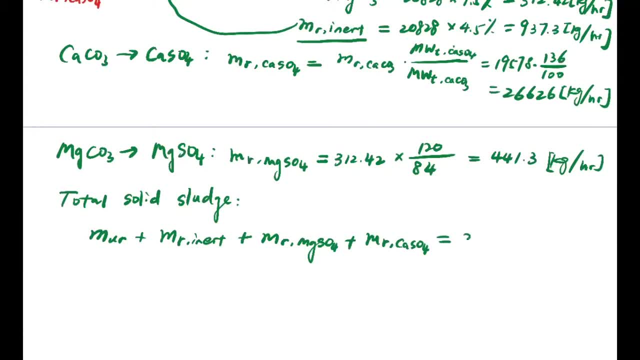 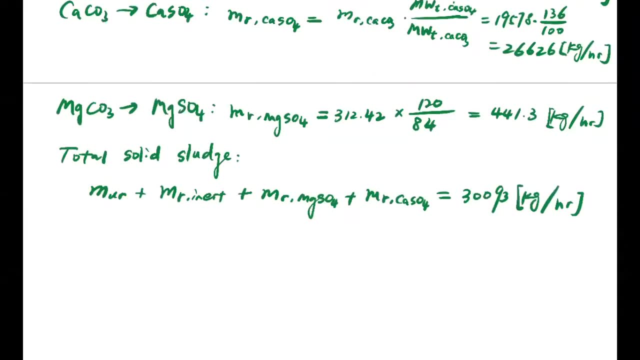 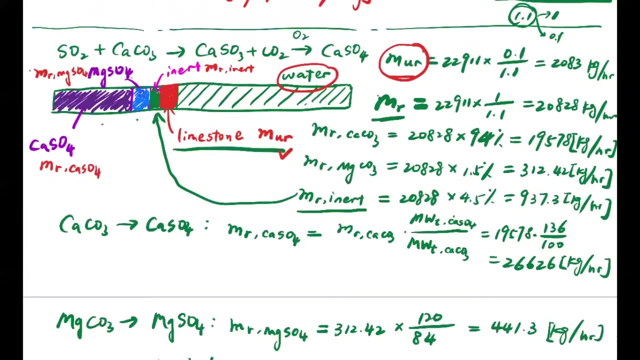 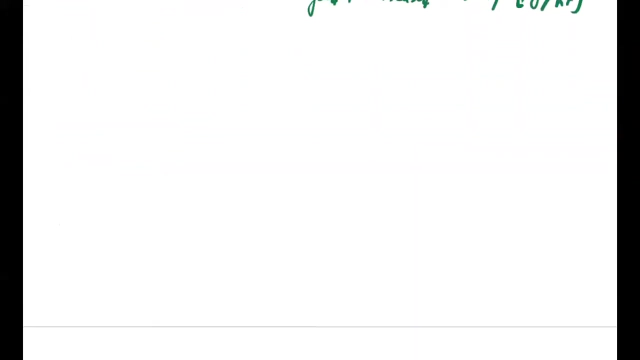 okay, so that's going to be three zero zero nine, three kilogram per hour, okay, so, finally, if we want to calculate the total mass of the sludge, we need to know that the solid actually just occupies 40 of the total sludge. water occupies 60, right? so what we need to do, 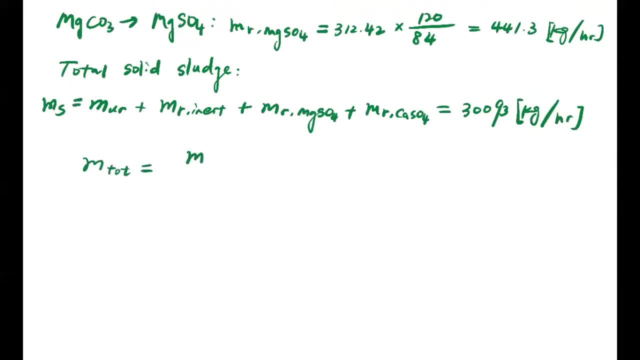 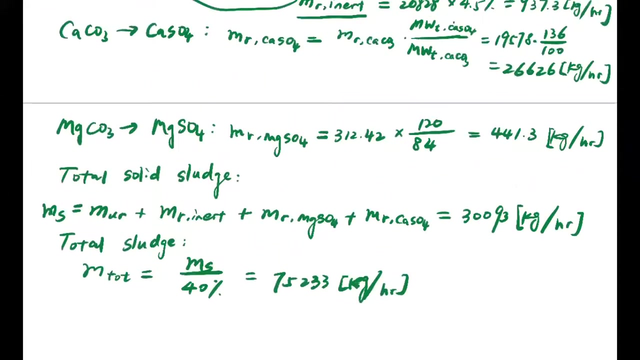 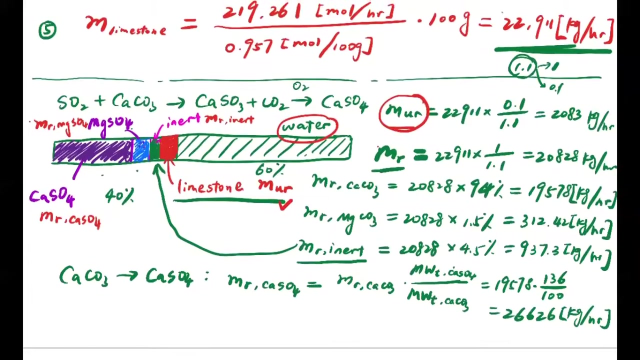 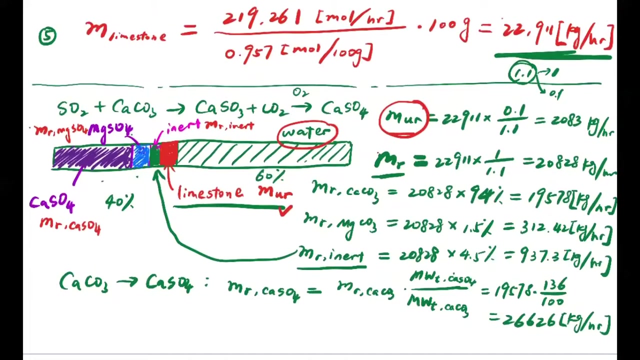 is to use the solid mass divided by 40, and that is 75233 kilogram per hour. okay, so this is a total sludge, but you can calculate the total mass by doing the same thing. all right, so this is. i think this is indeed a quite complex process, right? so you see that we use the 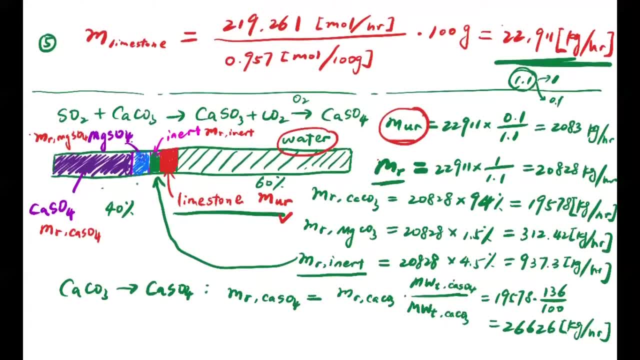 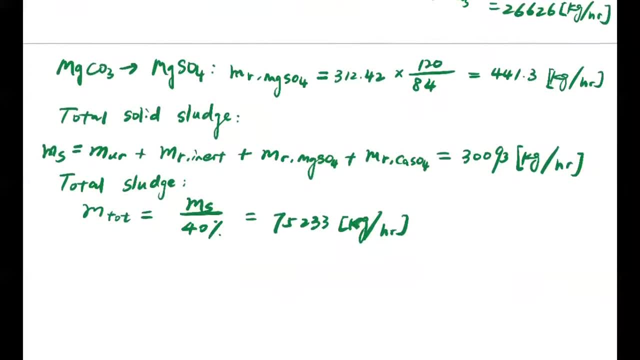 entire class to do these calculations. i'm not sure if you were able to catch me in typing the calculators there, but definitely in the homework and in the team project you need to go through these right. so, as we mentioned, we're just interested in two parameters for sulfur dioxide control. 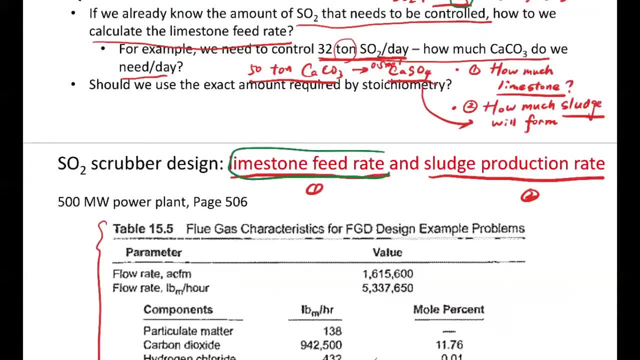 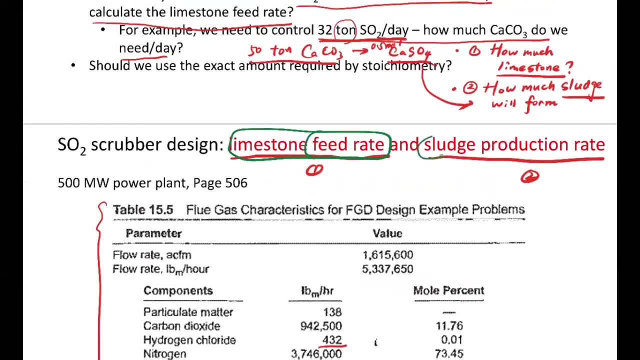 so one is the limestone feed rate, or i should say it's just the raw material feed rate. it can be lime, trona, limestone and so on, right, and the other is the sludge production rate, that is the product you generate from this reaction. okay, mainly because if we know these feed rates, then 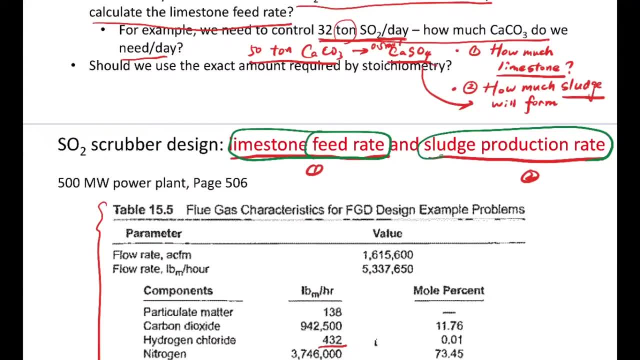 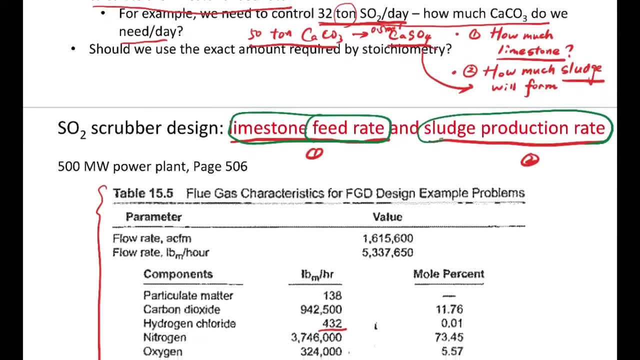 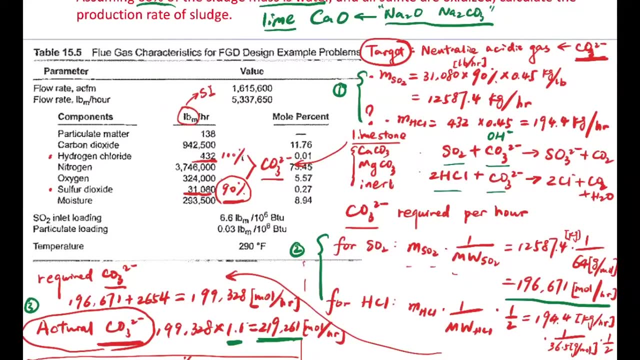 we can design other auxiliary systems or accessory systems to transport these raw materials and products. so i mentioned that for the feed rate we're using the carbonate ions as a link right to convert the amount of the acidic gases to the required calcium, to the required carbonate ions. 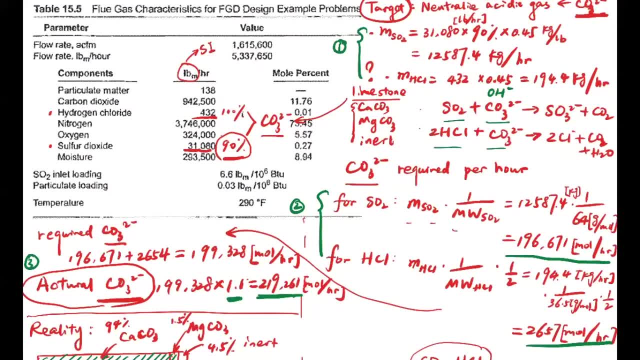 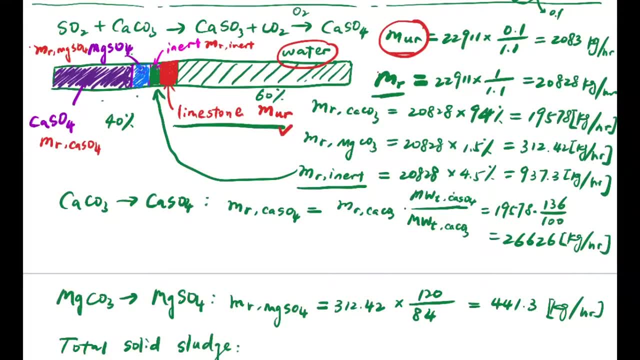 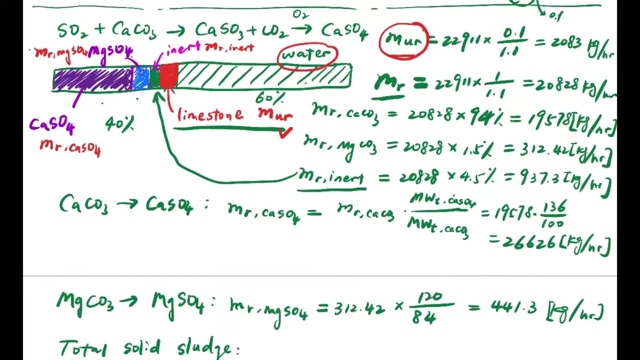 and then convert that required carbon ions into the limestone feed rate. and as for the sludge production rate, i think it's more straightforward if we can divide this sludge into different sections, right, and then just calculate the format of the production rate of each component one by one. okay, so again, we're trying to use this. 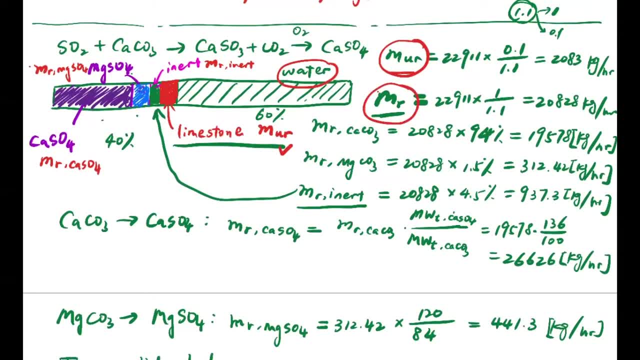 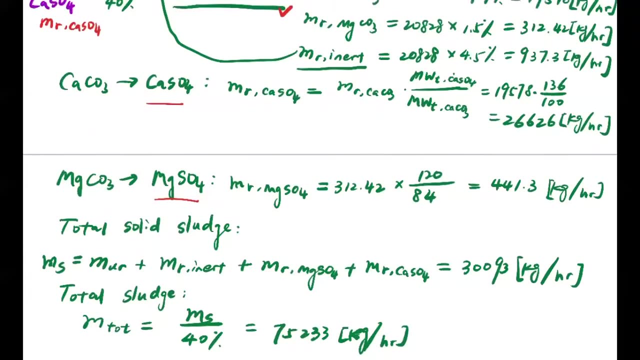 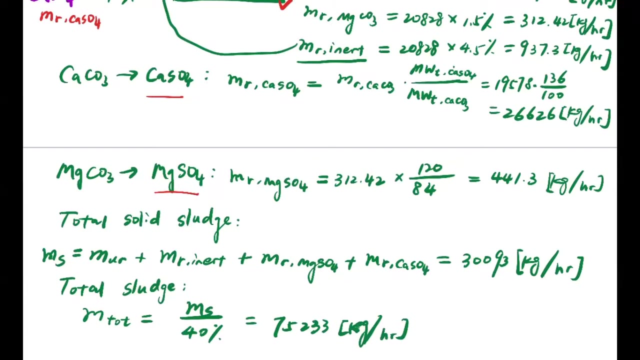 this reacted limestone right to convert it into the, convert it into the reacted calcium carbonate and magnesium carbonate and further into the calcium sulfate and magnesium sulfate. okay, so i would suggest that please do go through this calculation process and let me know if you have any questions. i know that there the complex can get very complicated here. okay, so if needed, 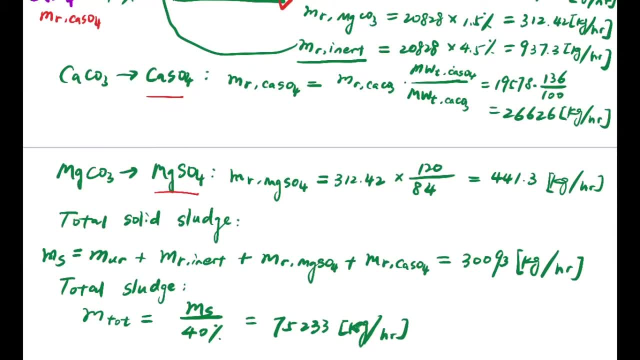 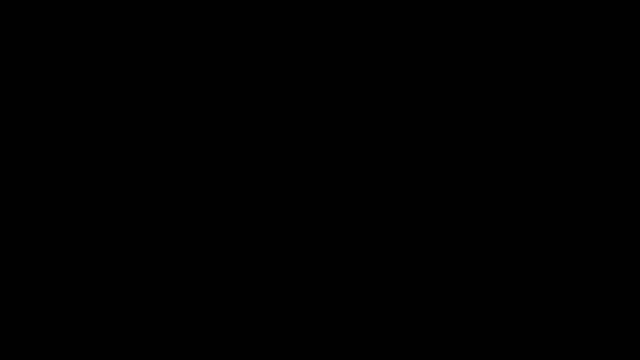 we can just go through this process again in our next class, but i don't think you guys can bear with all of these calculations here. so just let me know if you have any questions. that's all for this class.